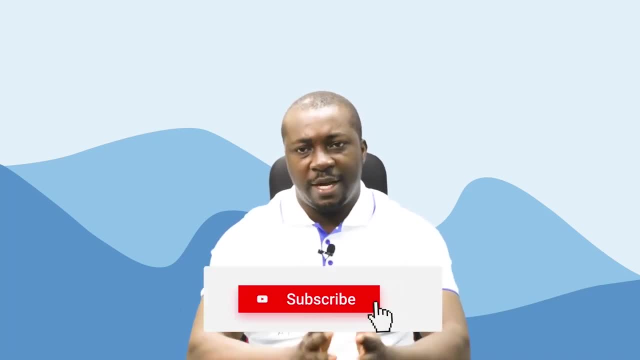 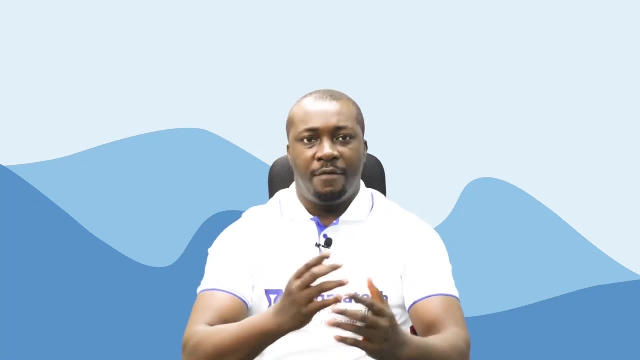 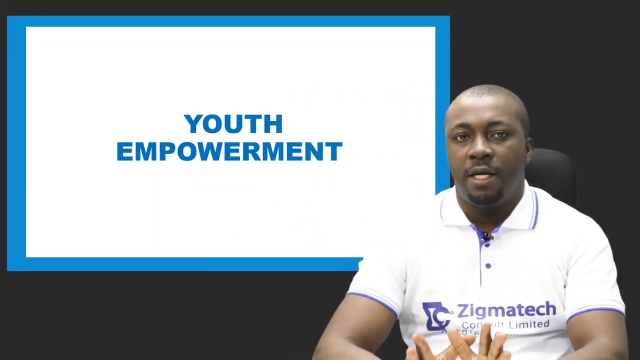 or Google Play Store. Please subscribe to our channel and turn on the notification bell so you don't miss our next video. Thank you, To be updated on new videos Ready for today's class. Okay, let's get started. In today's topic, we are going to look at the concept of youth empowerment. Of course, 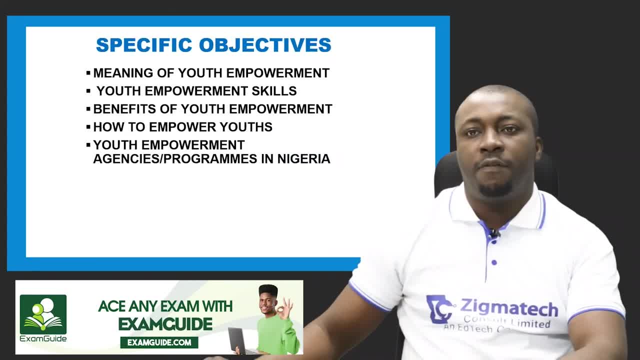 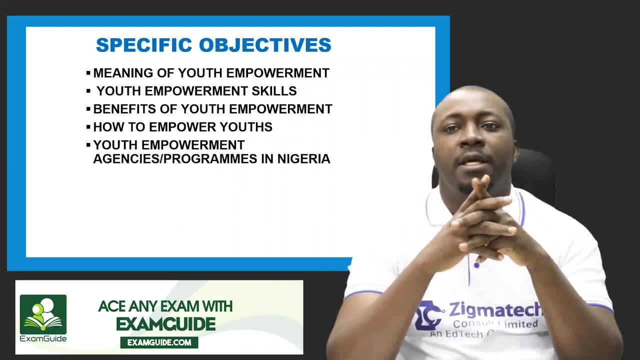 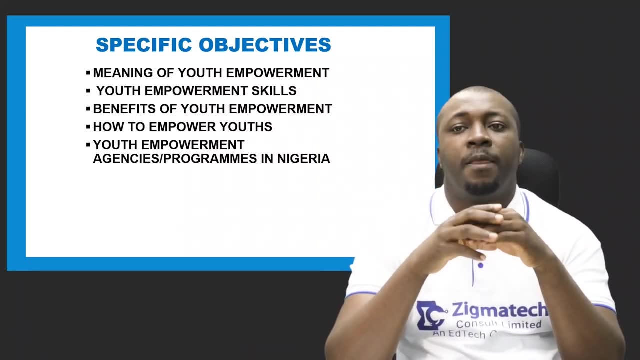 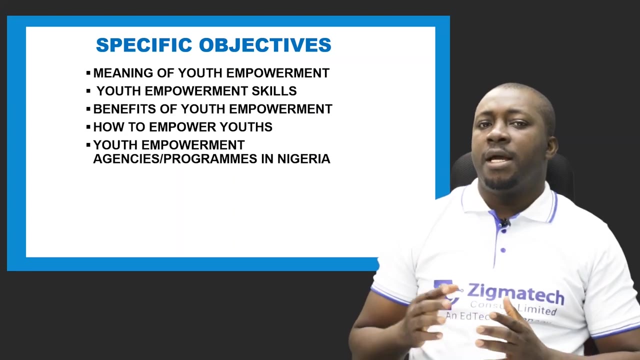 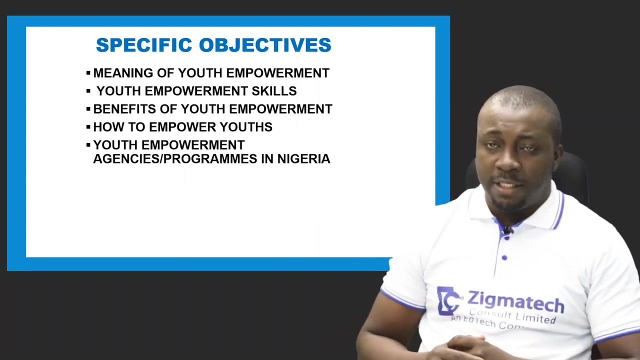 we need to be empowered Now. let's be specifically. by the end of this lesson, you should be able to define youth empowerment and discuss, identify and discuss youth empowerment skills, highlight the benefits of youth empowerment, Then discuss how to empower the youth and also discuss the youth empowerment agencies and programs of the government. 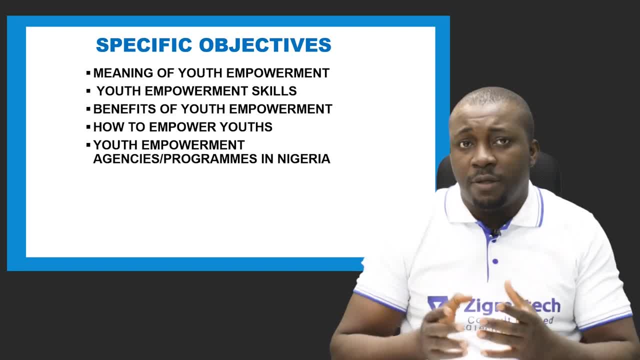 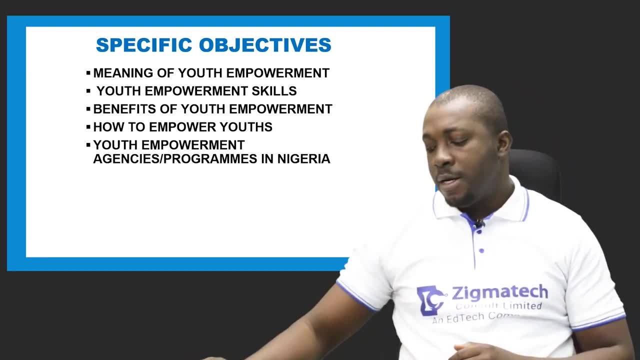 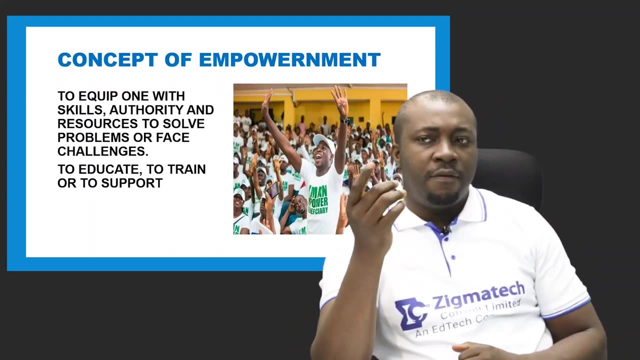 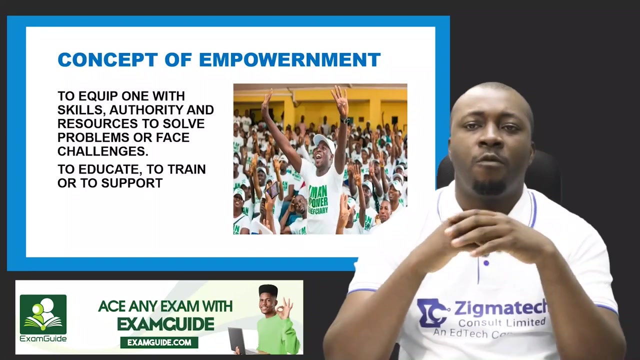 of Nigeria, So various programs that have been rolled out to actually empower the people, the youths in Nigeria. Now, let's start Now. let's first of all understand the concept of empowerment. What does it mean Now? to empower is to equip one with skills, with authority, give personal authority and resources. 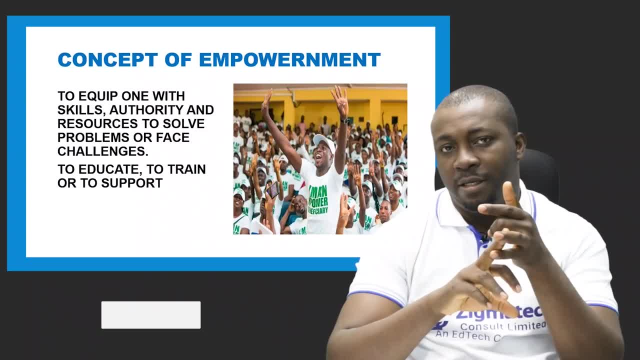 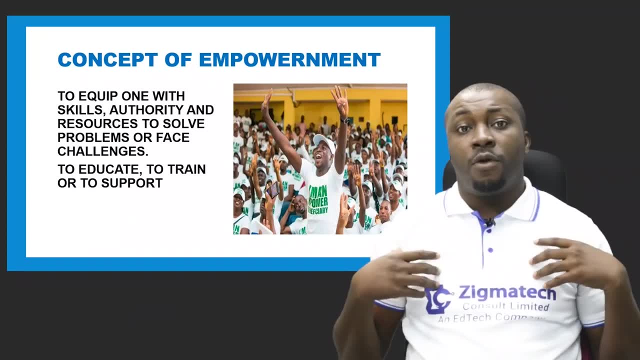 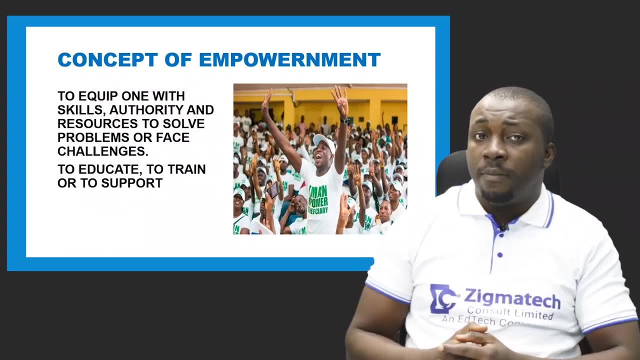 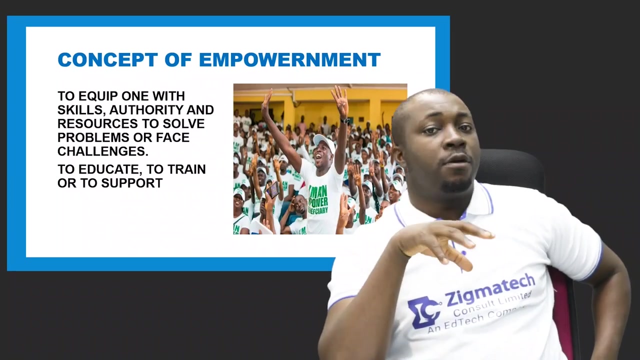 to solve problems and to face challenges of life. So it's all about equipping one with the necessary skills the person needs, the authority the person needs to act and also the resources to actually solve problems of life and actually face the challenges that life brings Also. 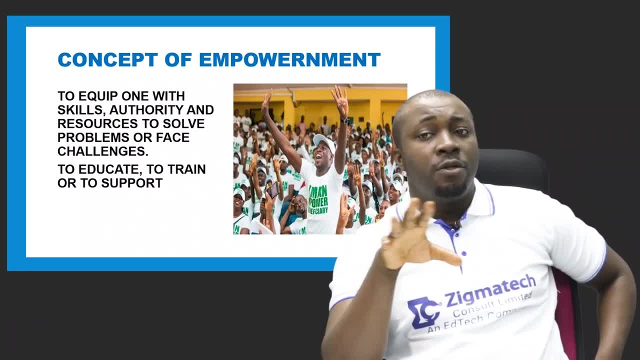 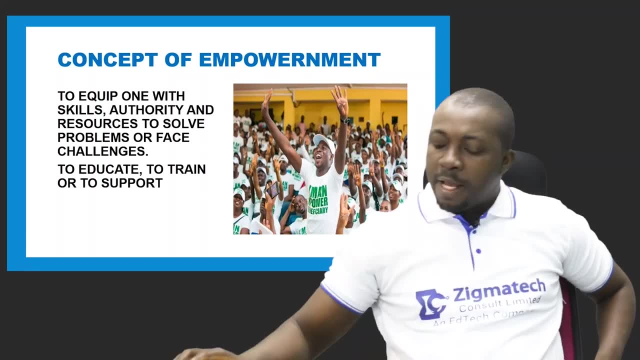 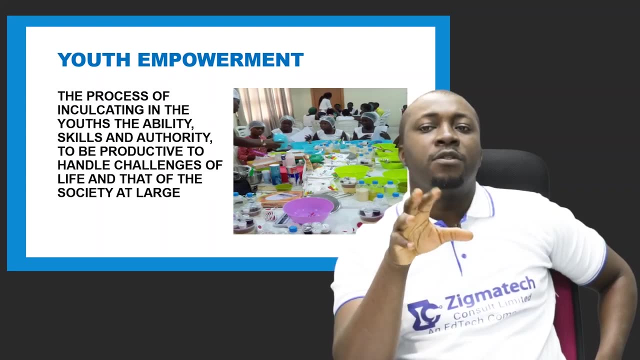 it involves to educate, to train and to give support to people. That is what it is: to empower people. Now let's look at the concepts of youth empowerment. Now. youth empowerment is a process of inculcating in the youths the ability, skills and authority. 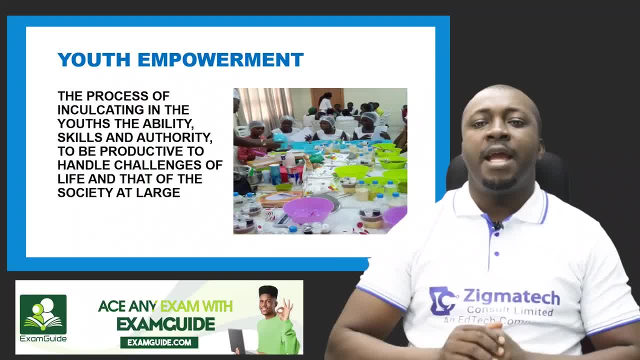 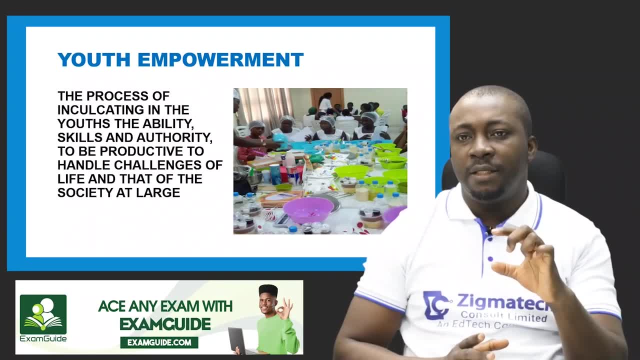 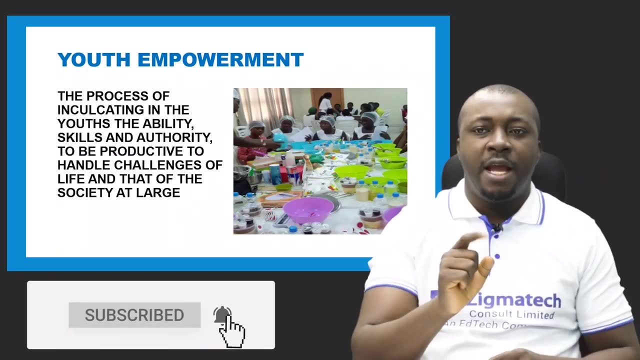 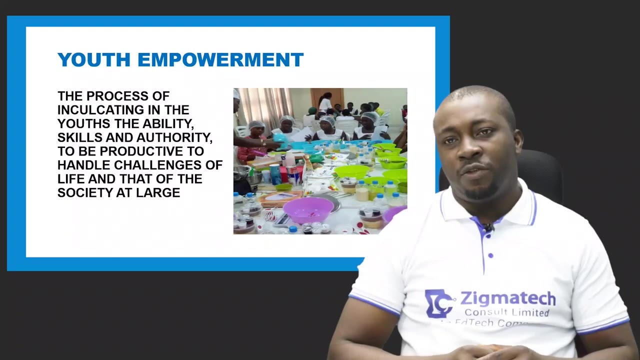 to be productive, to handle challenges of life and that of the society at large. So it's about giving the youths now the ability, the skills that they need, the authority that they need to be productive in life. It's about helping them to handle challenges of their life, their environment and the society at large. 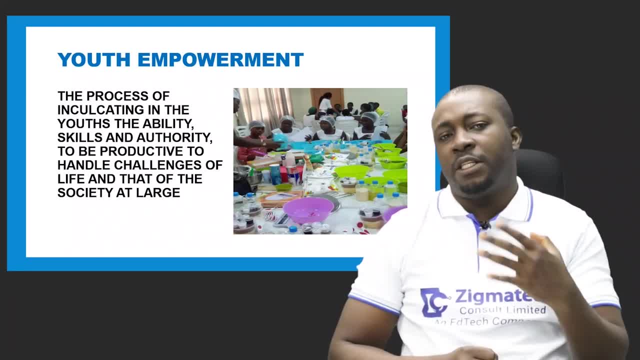 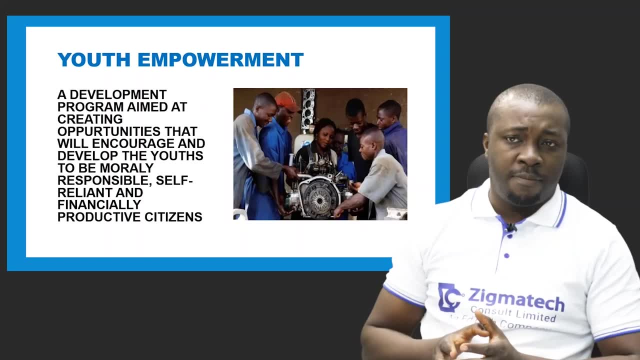 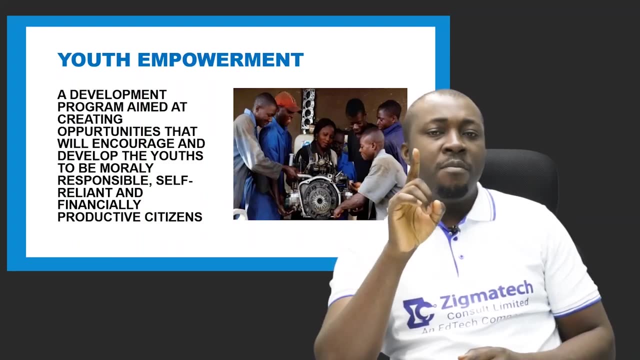 So youths are empowered to face challenges of their life and that of the society. It is also defined as a development program aimed at creating opportunities that we encourage and develop the youth to be morally responsible, self-reliant and not depend on people. 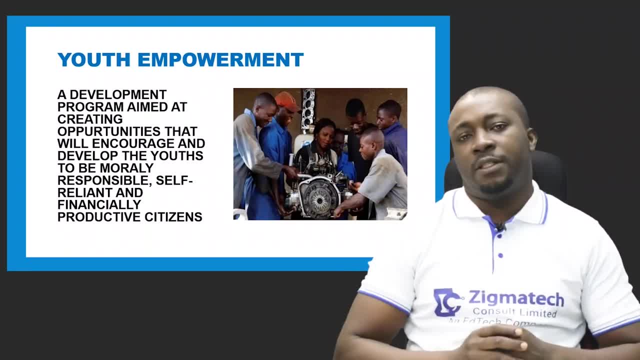 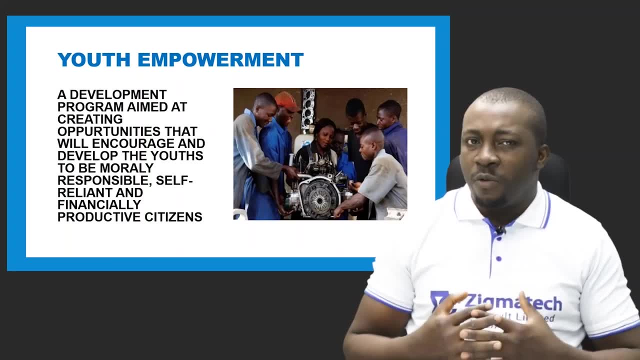 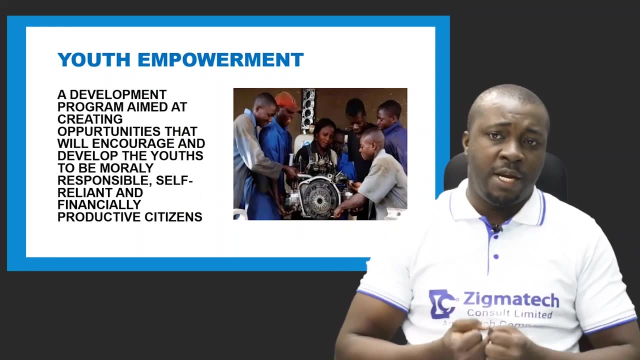 and financially productive citizens. so it's about programs that are developed to empower the youth, to equip them with the knowledge, to keep them with the skill, to keep them with the morals. they keep them with even the resources they need to be self-reliant to be morally responsible. 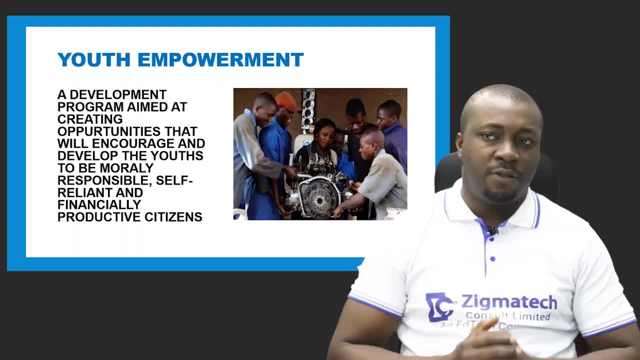 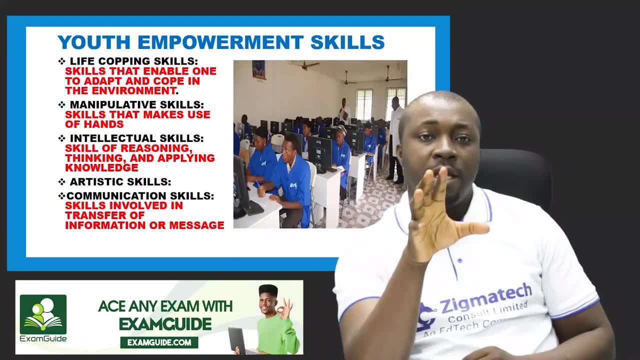 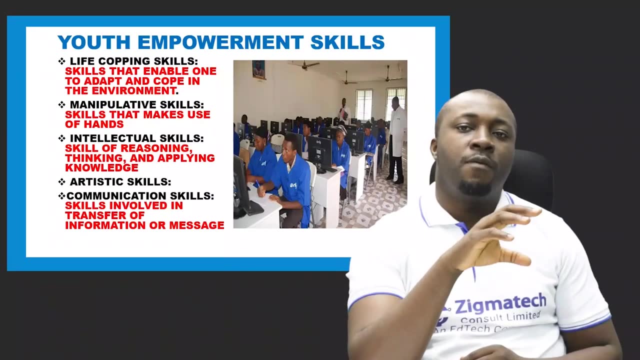 and to be financially stable in this society. now let's look at some youth empowerment skills, some of the skills that can be given to the youth through empowerment. number one is what we call life coping skills. now, when you talk about life copying skills, that skills enable one to adapt. 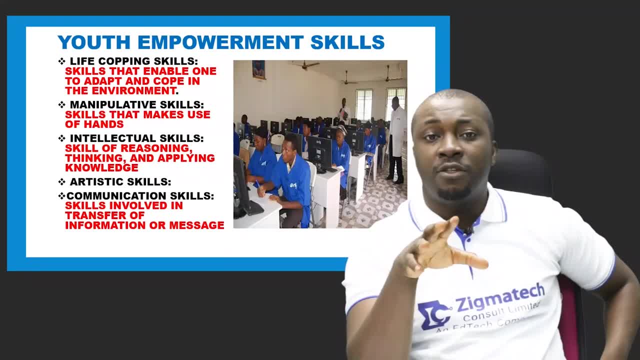 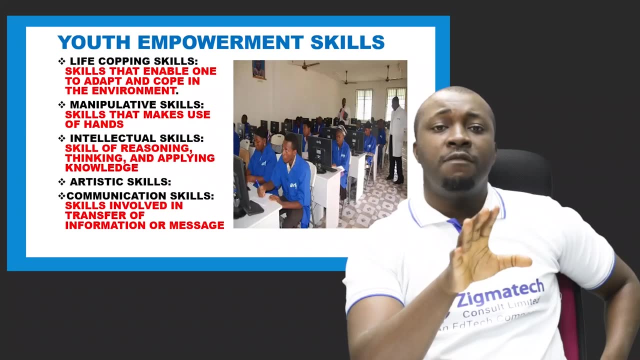 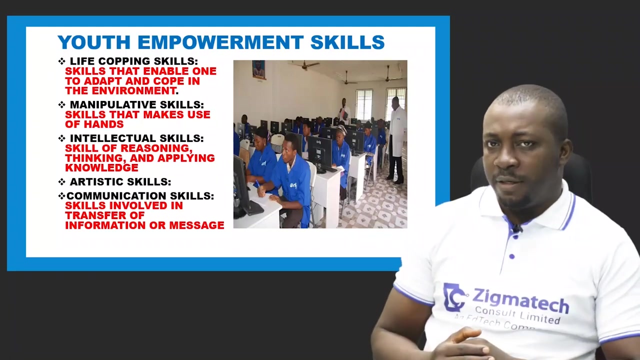 and cope with the environment. it's a natural skill that everyone should have. so it's about making one to be able to fit into the environment. one finds his or her self and how to adapt to all the vicissitudes of life that one we face. also, we have what we call the manipulative skills. now, manipulative skills are skills that makes use. 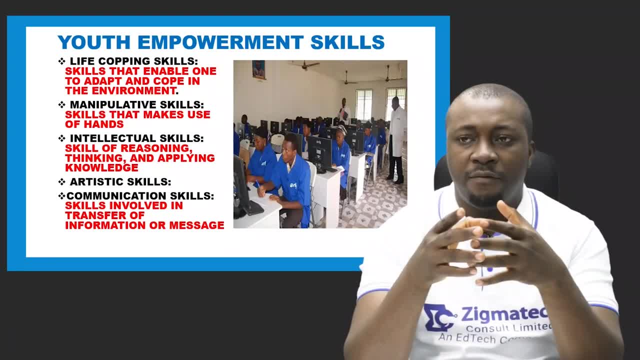 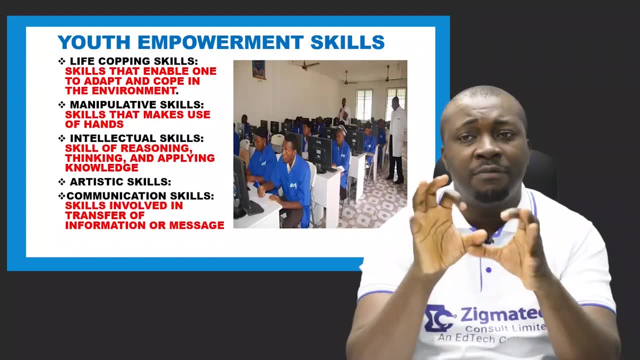 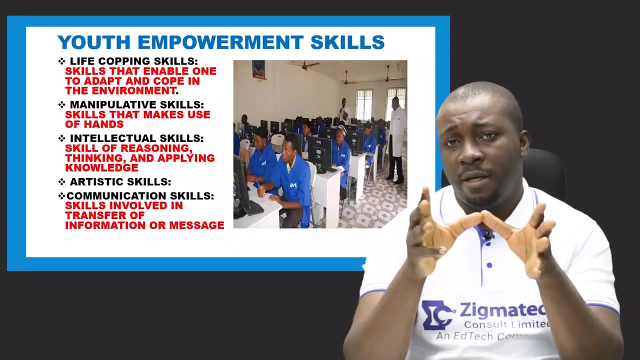 of hands to do things and in most cases, in vocational training, we get our manipulative skills. somebody who is into auto mechanics is into manipulative skills, so it's about using your hand to make things. so those that are involved- even those in bakery, some of them- have manipulative skills. 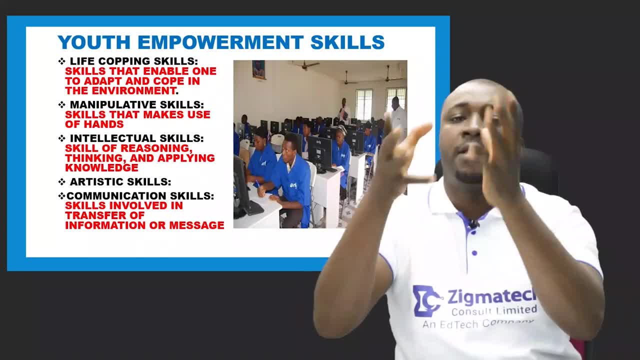 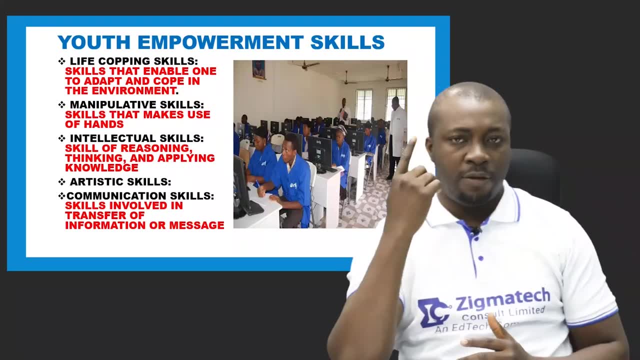 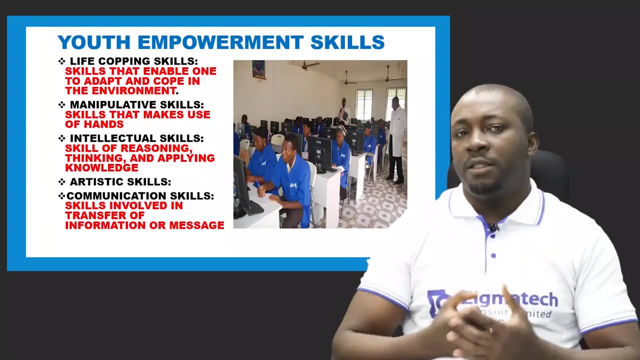 so ability to use your hand to fabricate, to make things, involve that manipulative skill. now we also have what we call the intellectual skills. now the intellectual skill has a skill that boosts reasoning, thinking and application of knowledge. now these intellectual skills are mostly gotten in schools. 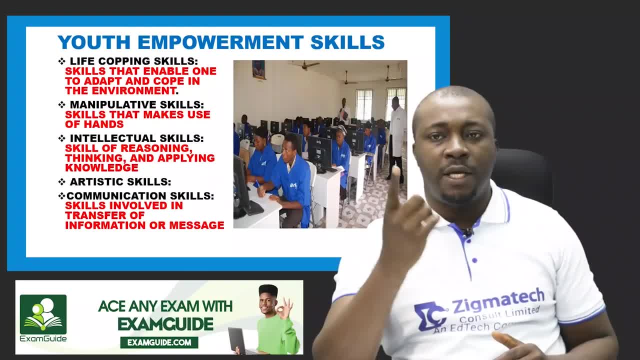 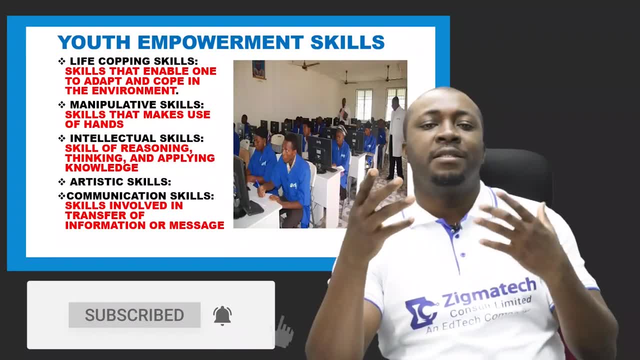 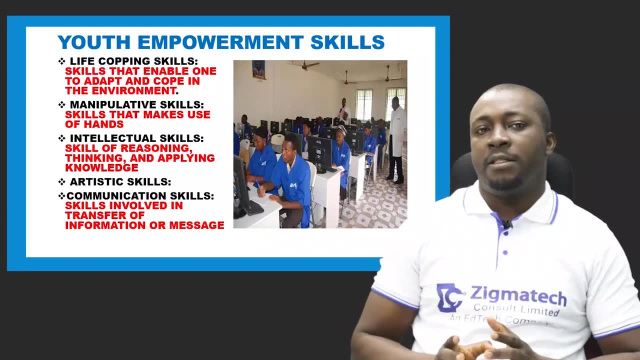 it boosts your analytical thinking, your logical thinking. so it's about intellectual skills, it's an academic skill. now we also have artistic skills. now, in artistic skills we have those that are into pure and find us so that can draw, paint, make things, make things, create beautiful things, those things we use to absorb science, some resources, for example. 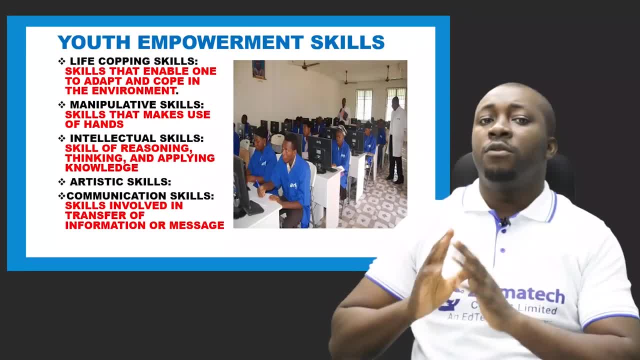 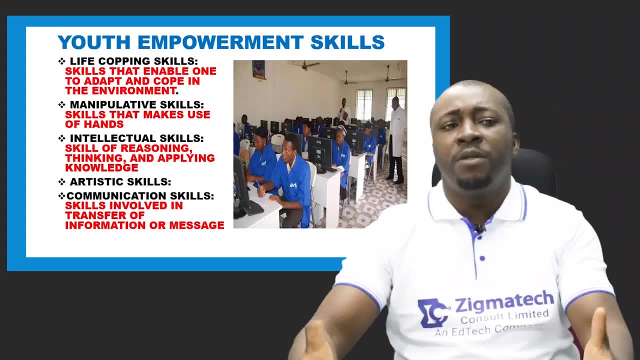 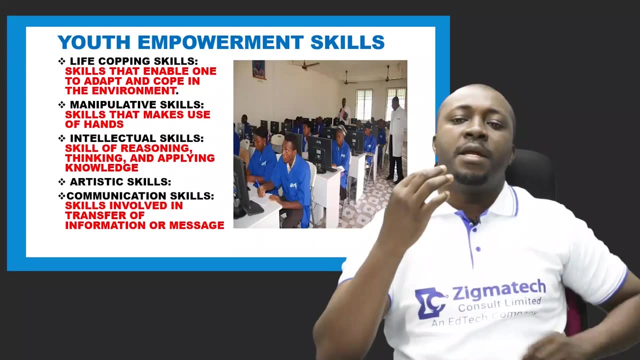 things, those that are into aesthetics, And also we have those that are into entertainments. You have the actors, you have the actresses, you have the musicians. These people are into artistic skills. Now we also have communication skill. In communication skill we talk about. 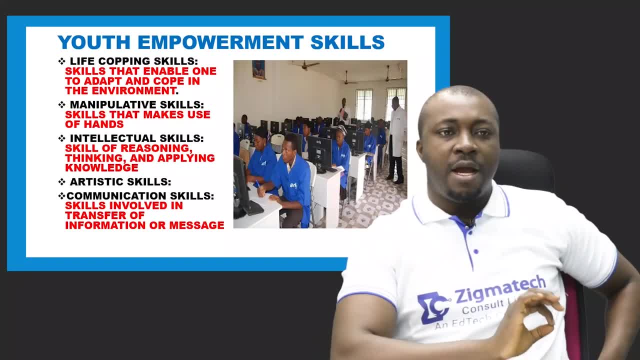 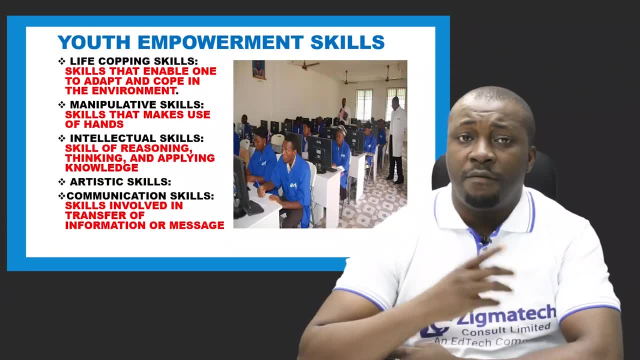 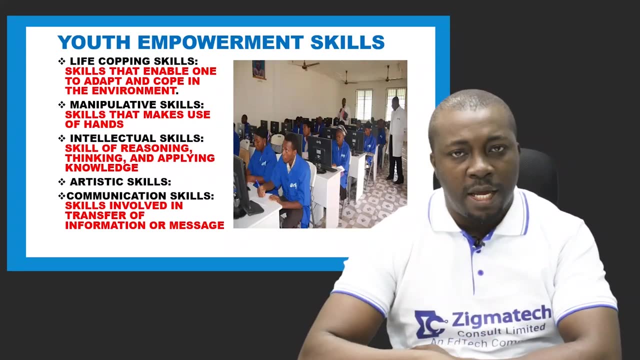 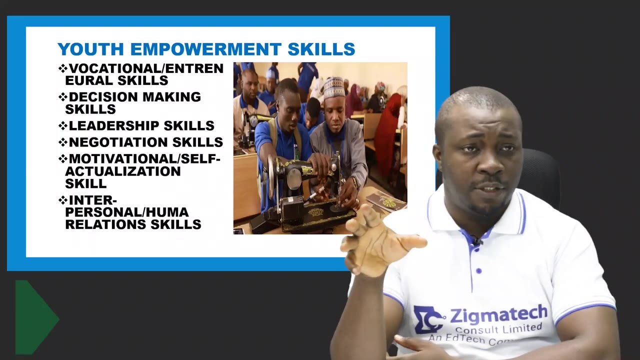 skills involved in the transfer and even research of message. So it involves transferring messages, it involves receiving messages, skills involved in enhancing proper means of communication or information dissemination. We also have what we call vocational or entrepreneurial skills, And that is why a youth empowerment, or people open what we call Vocational Training Center. 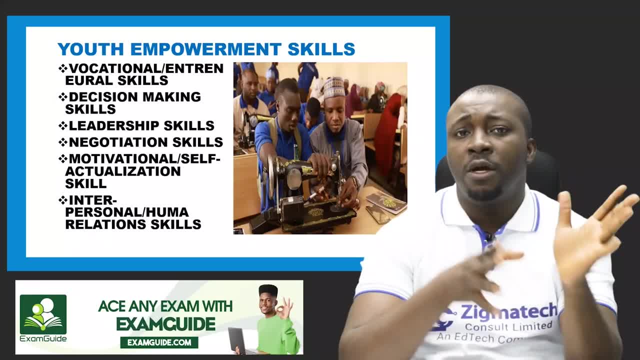 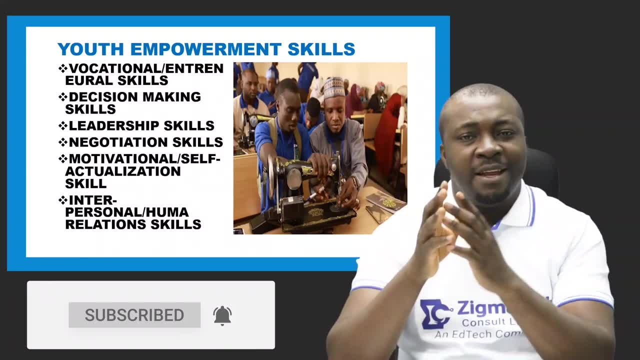 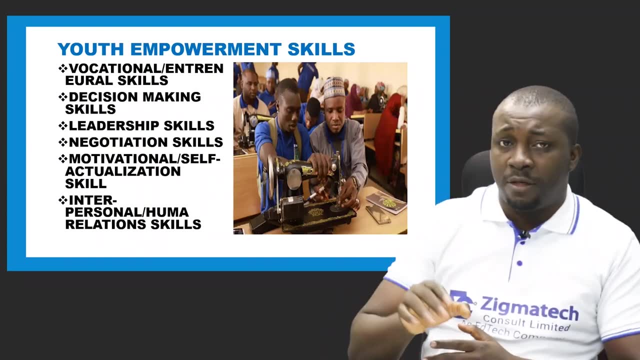 to train people to go into one vocation or the other. we also have decision-making skills- skills that enable people to take their right decision at every point in time. it's not everybody that knows how to take the best course of action when you have choices, so it's also skilled by enables 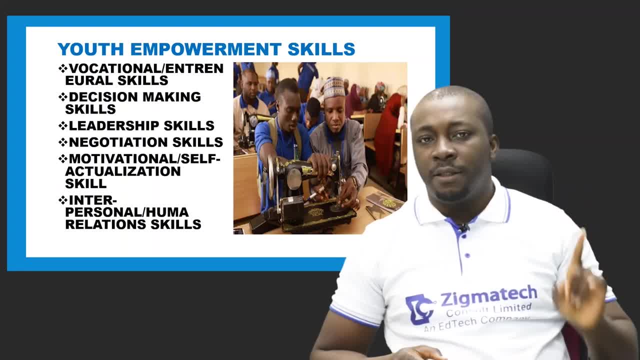 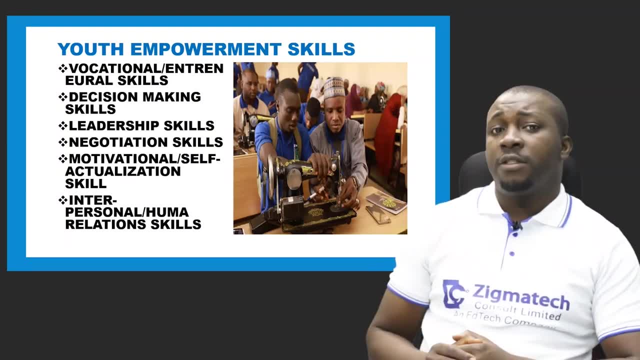 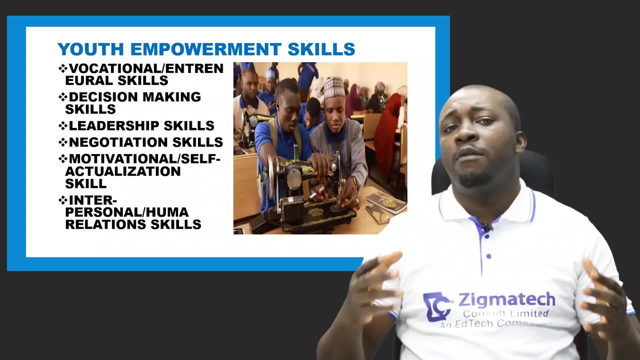 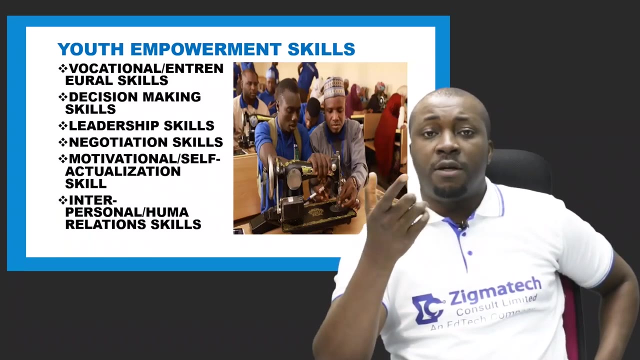 one to always, at every point, take the right decision. we also have leadership skills. youth are empowered with leadership skill because they are leaders. they should be the leaders. so leaderships get a people one on how to influence people, how to lead people. we have negotiation skills: negotiation skill- how to bag in, of course, if you come to conflicts, which is 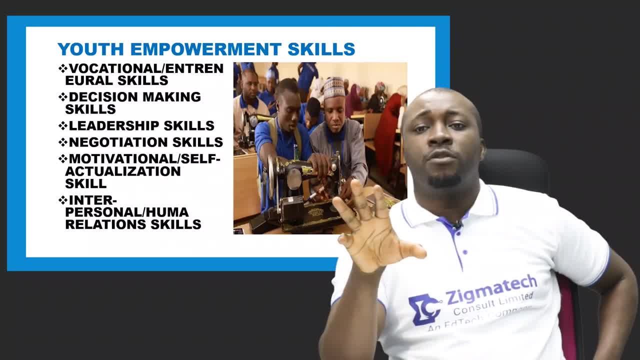 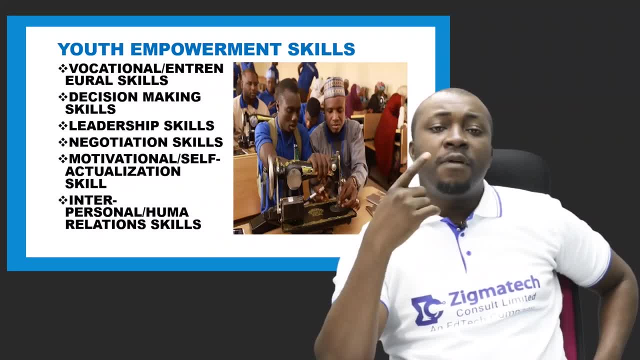 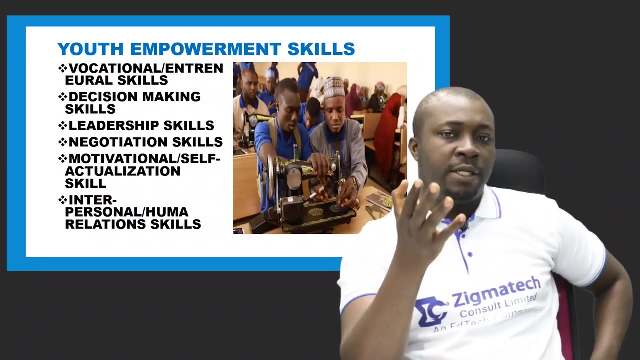 a, the unavoidable aspect of our social life. negotiation skill is important in managing conflict, even in businesses. we talk about negotiation in workplaces. we talk about in every aspect of social relations. we talk about negotiation skill. then we have motivational and the self actualization skill, skill that enable you to motivate yourself to work towards actualizing. 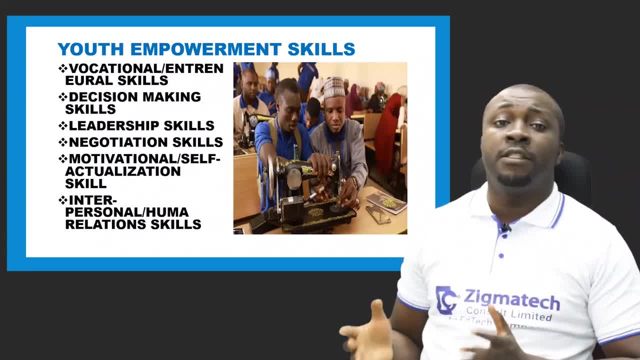 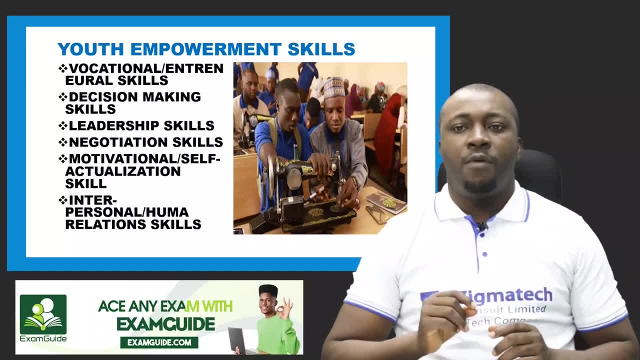 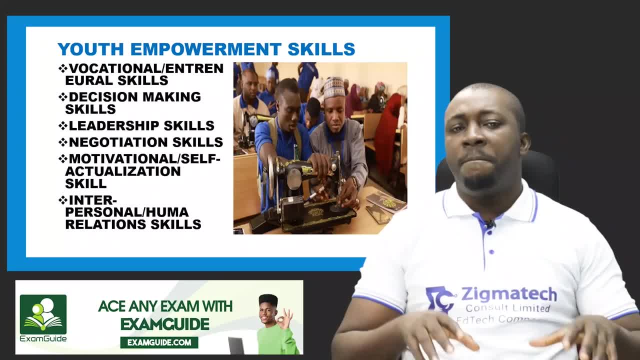 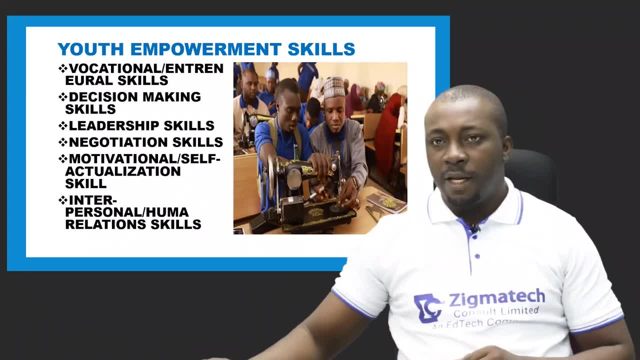 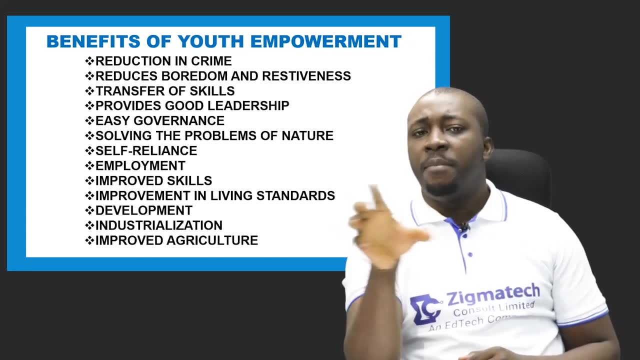 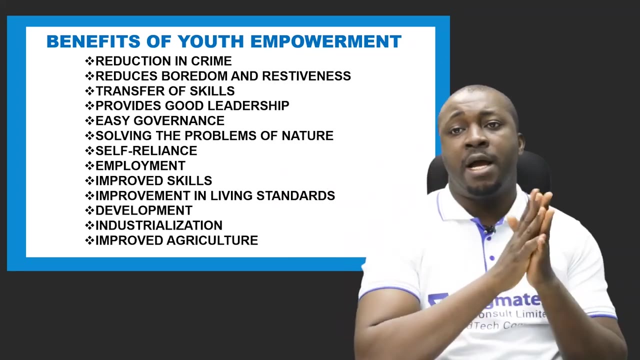 these are the skills that promotes you to have better relations with other people around you. so these are the youth empowerment skills. now let's look at benefits of youth empowerment. what are the things, the benefits derived? what are the importance of youth empowerment? one reduction in crime when youths are empowered, especially in such a way that they engage. they are engaged in. 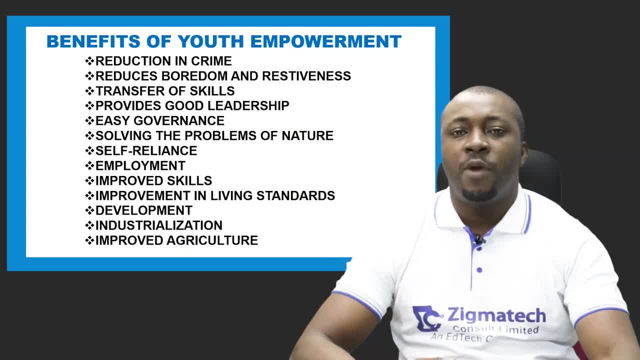 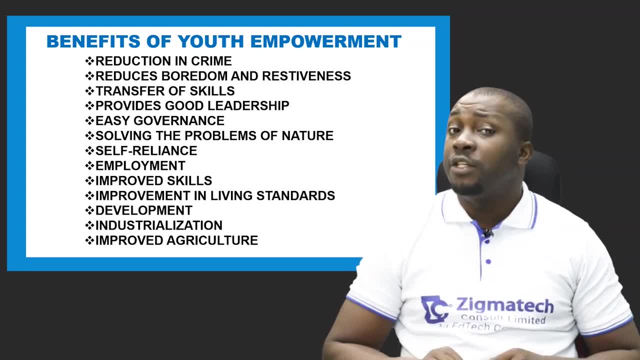 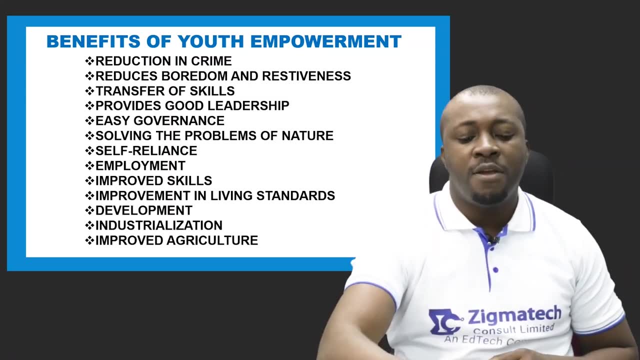 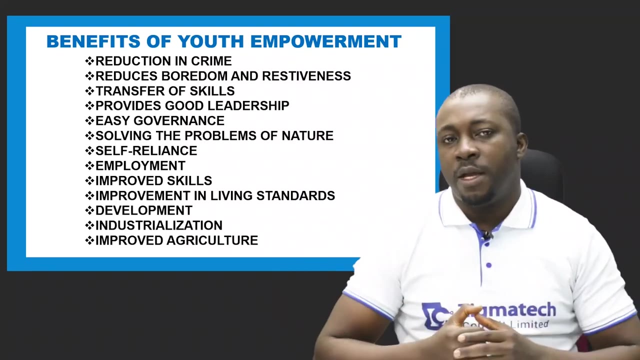 productive Ventures. of course it will help and reduce crimes drastically in the society because they see an ideal manager is a devil's workshop. so when people are not doing anything they can engage in home and off crimes. and that is why youth empowerment is important to help to reduce crime, because people the use you be engaged. 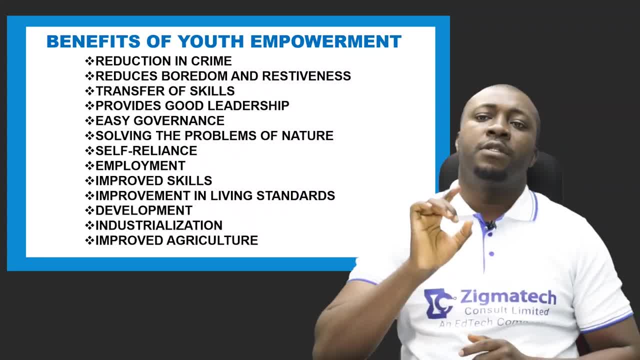 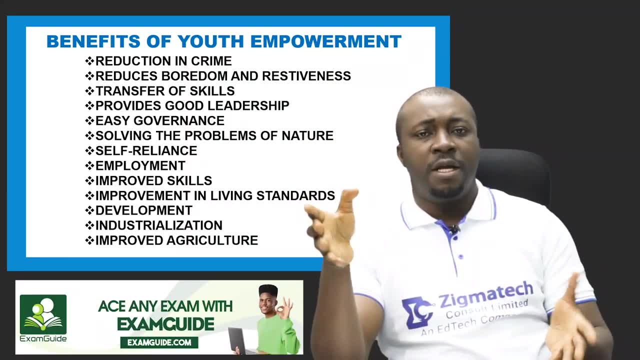 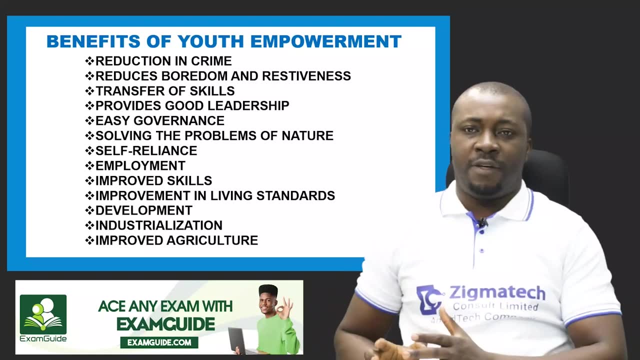 and will not indulge in crime. it reduces burden and restiveness. when people are empowered, they will not feel bored, they will not feel idle, they will not feel restless because they are active, they are involved in. in fact, coming back home will be that you have retired from the 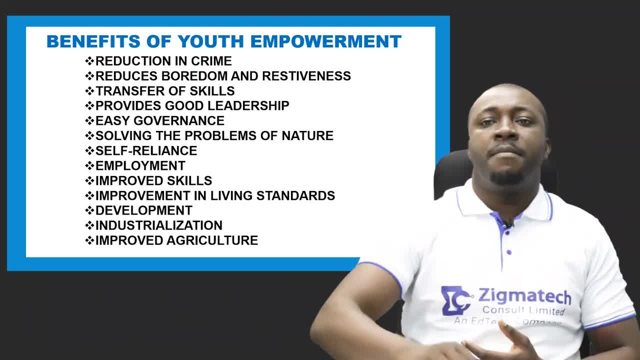 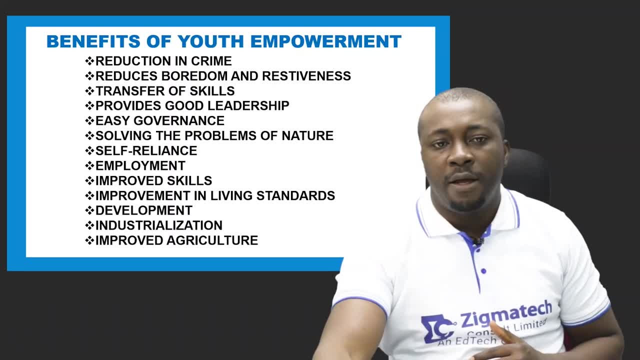 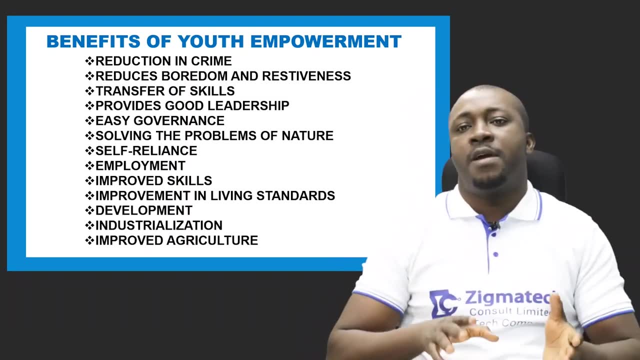 day and you want to rest. youth empowerment leads to transfer of skills, skills that transfer from one person to another through the process of teaching and learning, training on one skill or the other. so you see the transfer of knowledge and skills from one person to another and people acquire skill that. 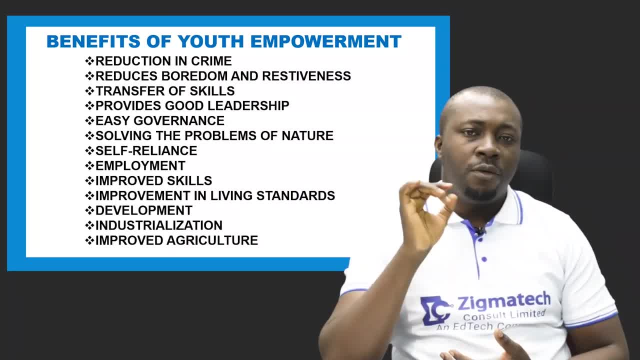 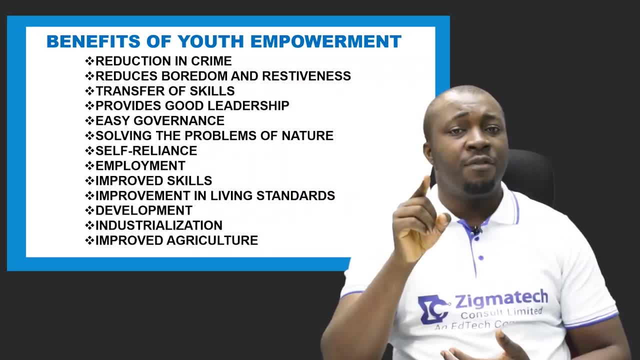 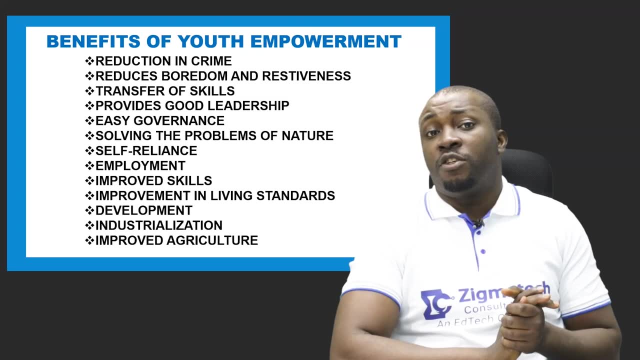 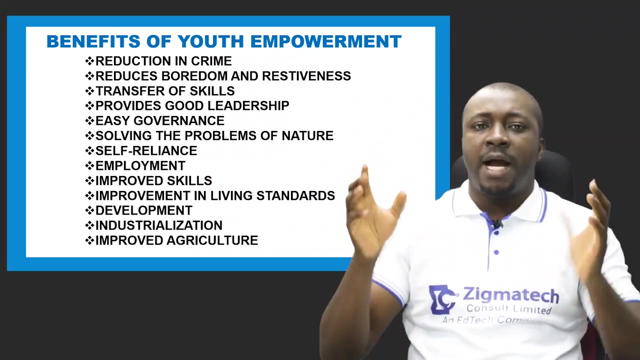 are being fed to them. it provides good leadership when youth are empowered, given leadership training. of course we have good and better and responsible leaders in our society because these people have been trained to lead, then there'll be easy governance. when people are empowered, engaged in productive ventures. 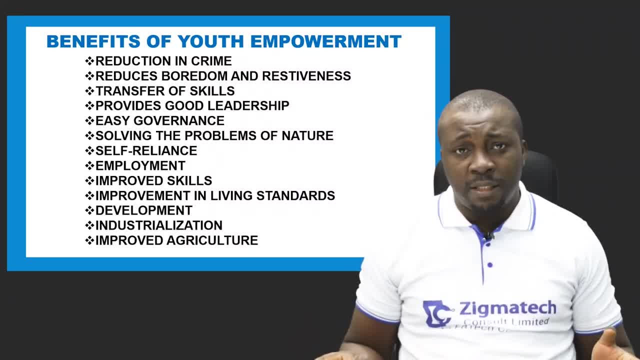 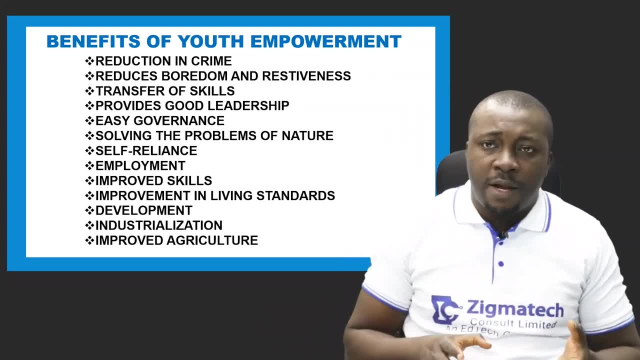 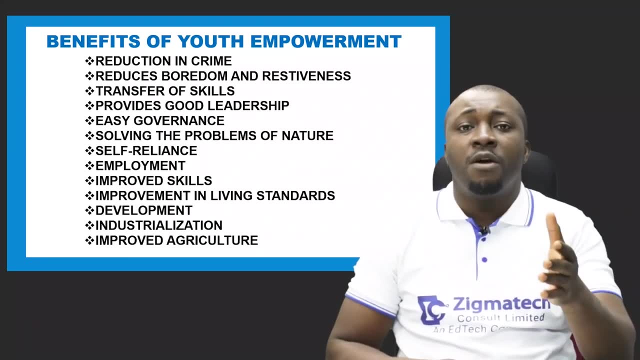 crimes will reduce and governance becomes easy. the government will not be spending more money to combat crimes and also repair the effects of crime. government will think of: okay, what are other basic amenities we can do to make this society comfortable, more comfortable for the citizens also. so it 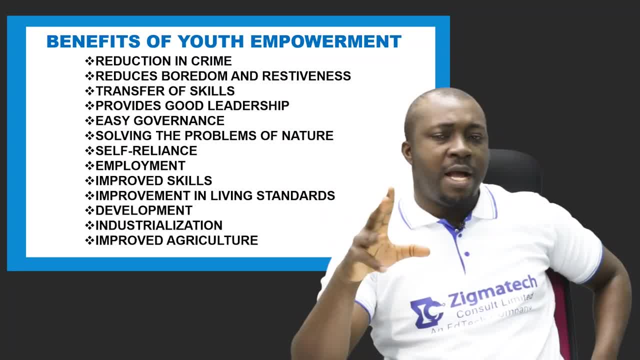 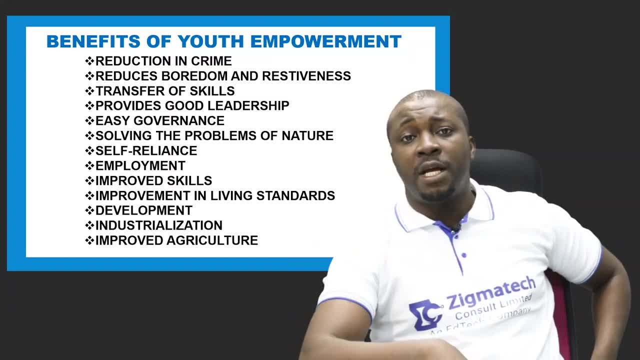 makes governments easy in the society when youth are empowered and of course, there'll be more revenue to the government because more people are engaged in productive ventures and they're paying tax to the government. also, solving the problems of nature is one of the benefits of youth empowerment. when youth are empowered, it equips them to. 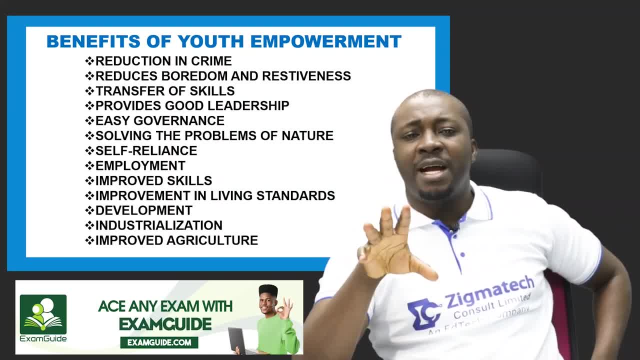 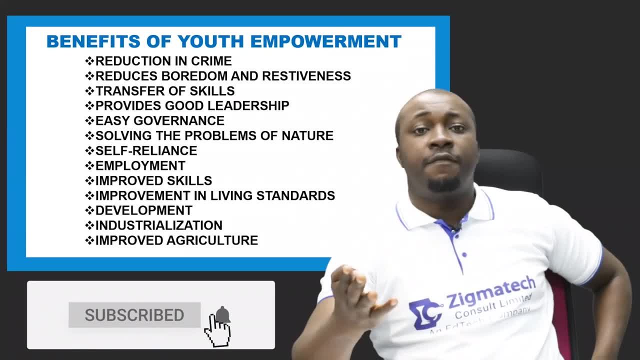 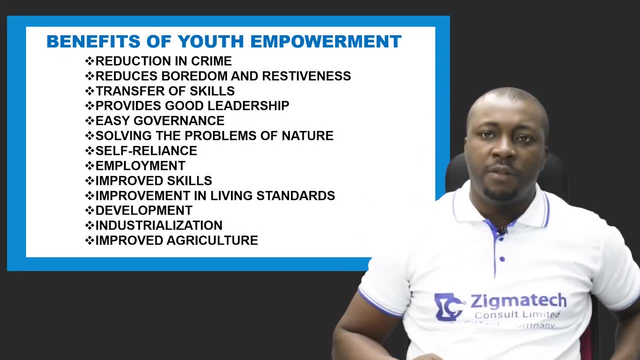 solve the problems of nature, because we people encounter one problem or the other in their lives, so it helps. it could be financial problems, it could be any other form of problem, so empowerment can help them to solve their problems. then it brings about self-reliance- self-reliance on the part of the 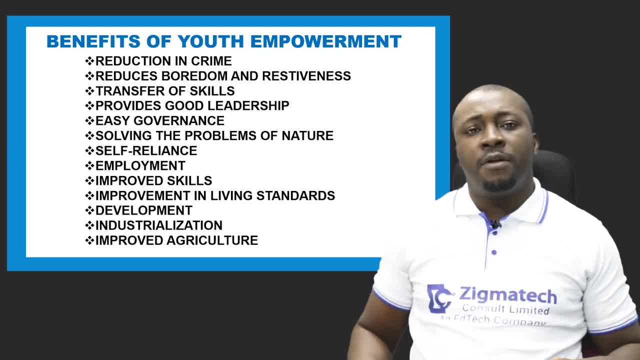 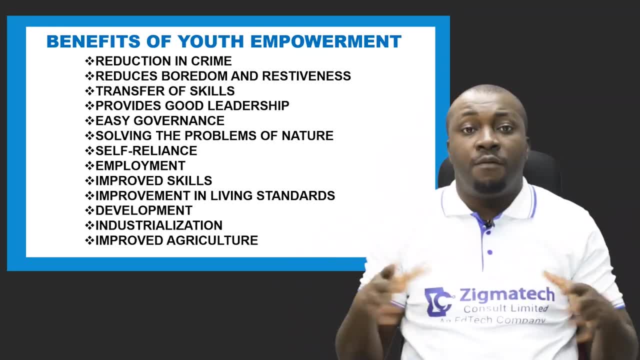 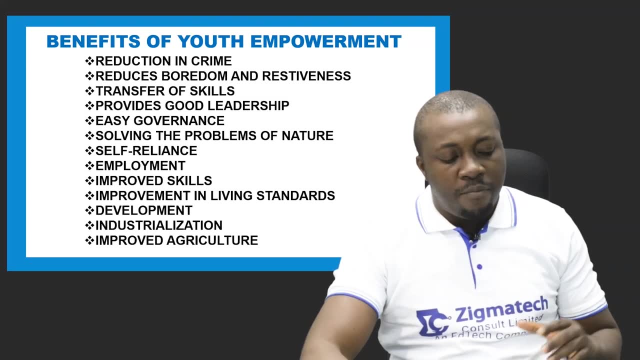 individual first. you are, you rely on yourself, your don't actually depend on people. you work for your own, you make living for yourself. on the part of the nation, it is the part way to self-reliance, because when people are endorsed, we can talk about industrialization. 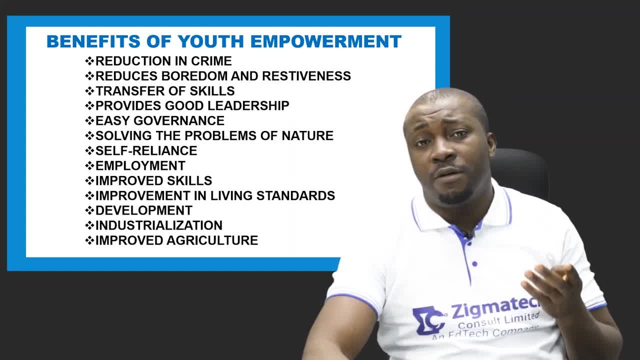 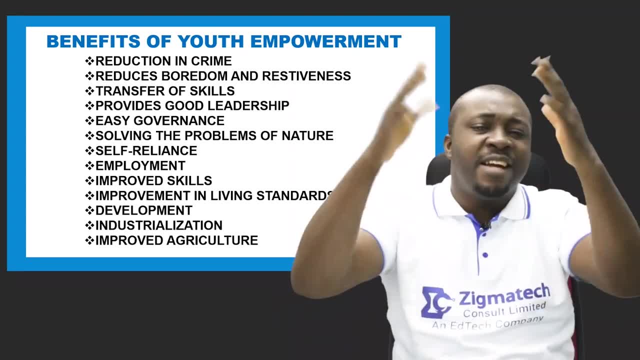 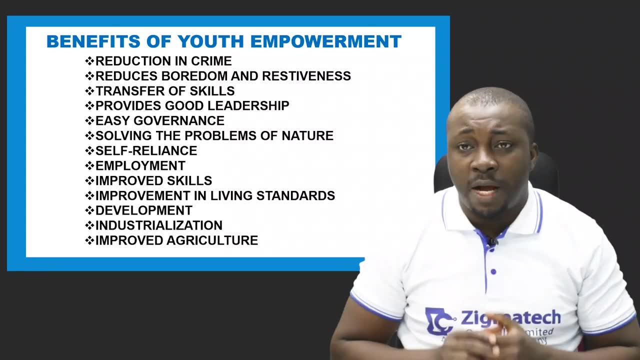 When you boost people's entrepreneurial skill, vocational skill, manipulative skill, of course, it will lead to people creating jobs and not mere job seekers, And with that industrialization can grow and the nation can become a self-reliant nation. 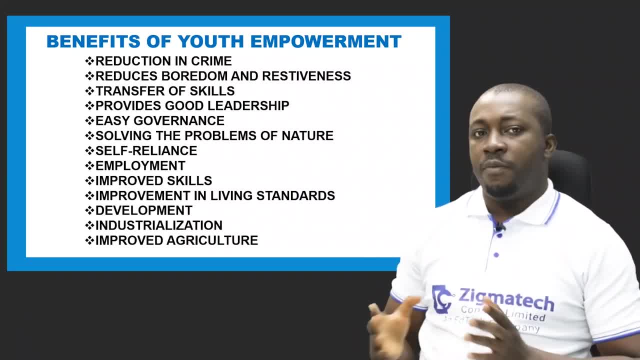 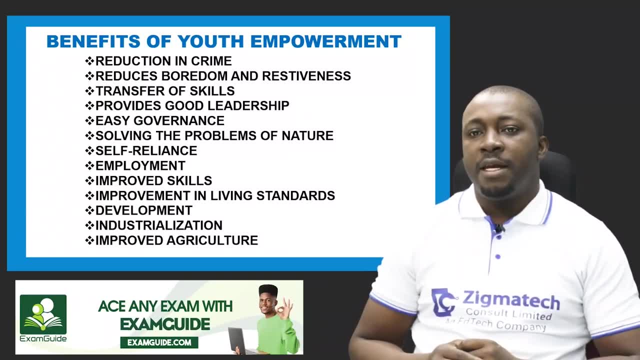 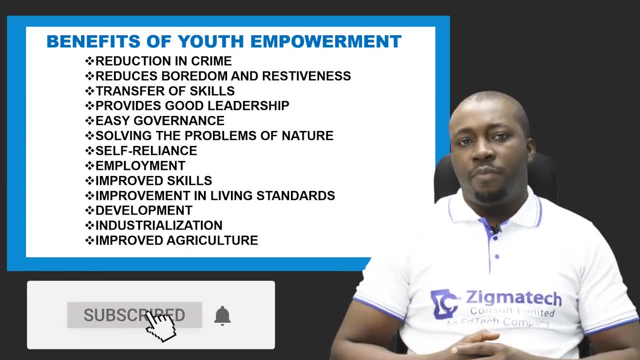 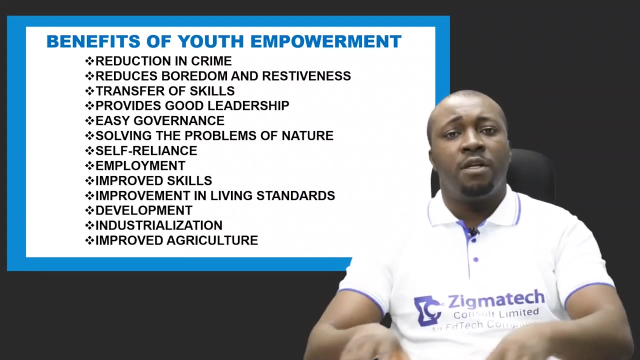 It brings about employment. When people are empowered, involved in one productive venture or the other, of course, they are automatically employed And it boosts employability of citizens, especially the youths who are being empowered. It brings about improved skills. People have skills, acquire skills. through empowerment, We'll be able to acquire skills to do one thing or the other, solve their personal problems. 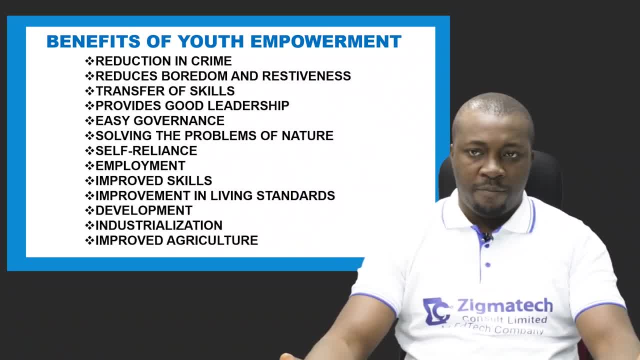 Also, it improves standards. It brings about improvement in standards of living in the sense that when people are empowered in such a way that they are engaged in one productive venture, one work, one occupation, one vocation or the other and are able to comfortably meet their basic needs, of course the standard of living of the individual, even the country at large, will improve. 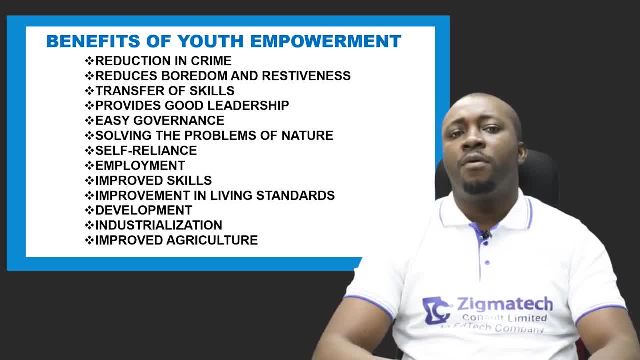 It brings about development. When people are engaged, when the youths are adequately engaged, of course the gross domestic product, the gross national product of the country will improve. Government will have more revenue, So of course, automatically the country will improve. 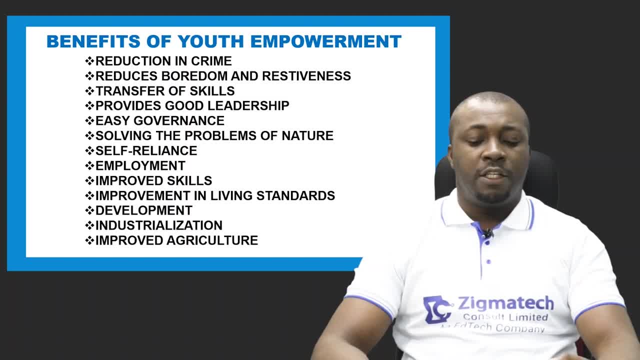 It brings about industrialization. That is why in youth empowerment, vocational training, manipulative skill are emphasized. So this will bring about industrialization, because when people learn certain things and begin to do it- their own, of course- such can grow into a large-scale industry. 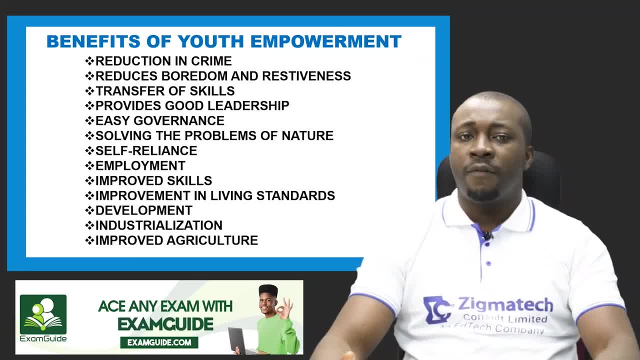 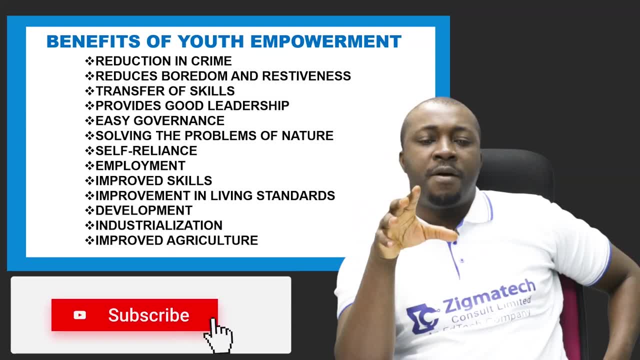 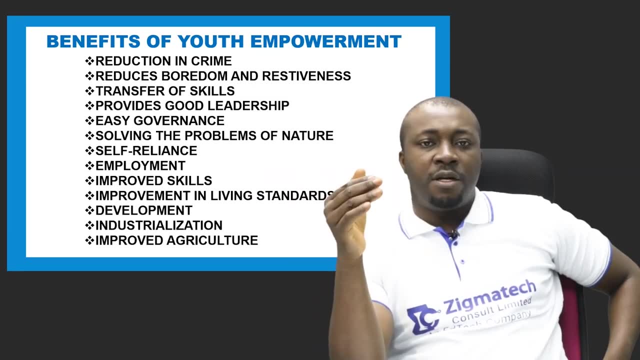 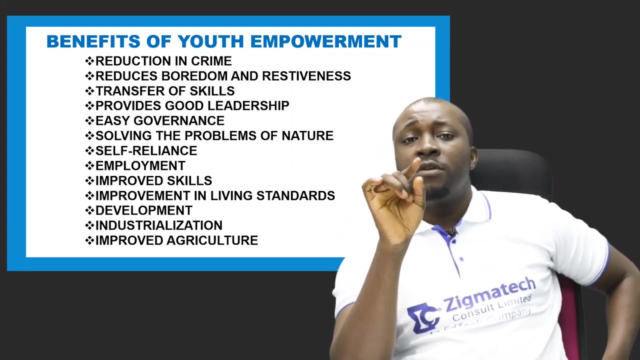 So it can boost industrialization, That is, the growth of industries in a particular country. There will be improved agriculture When people are empowered, especially in the area of agriculture, which most youths, many youths, are neglecting Because they don't see, especially in this part of the country of the world, in Nigeria. you see that youths, they don't see meaning. 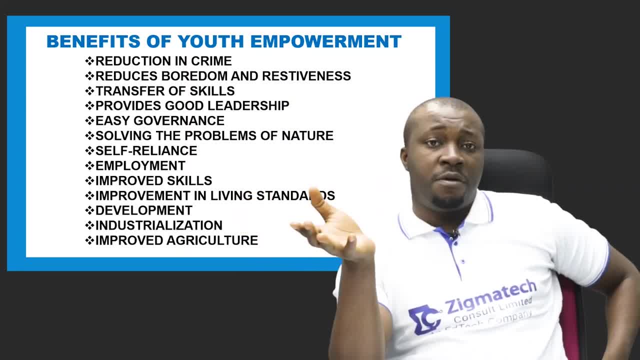 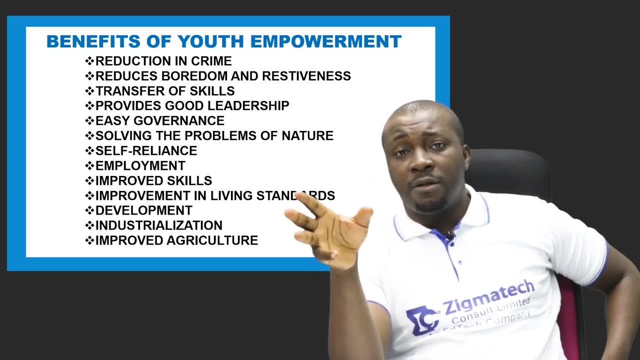 They don't see prospect in agriculture. People favor more of white-collar jobs. They don't want to talk about their villages. They don't want to talk about agriculture. Of course, empowerment in the area of agriculture, like giving free fertilizer or subsidize the cost, 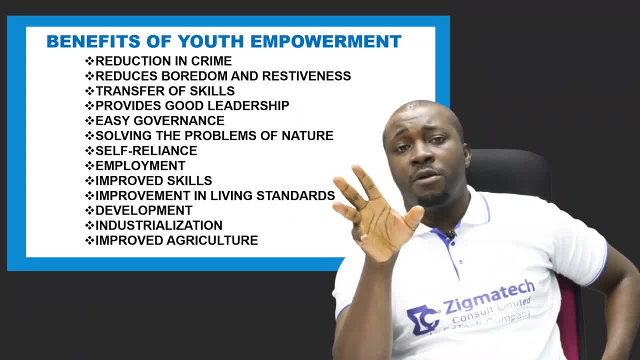 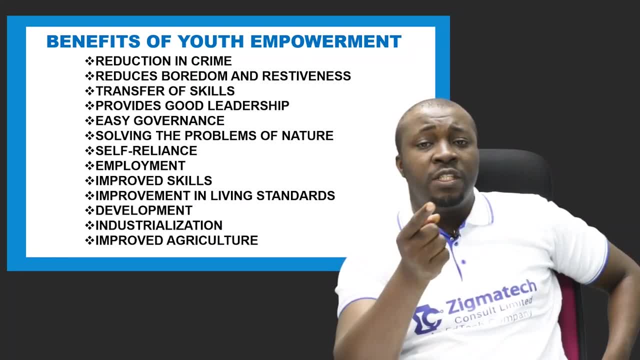 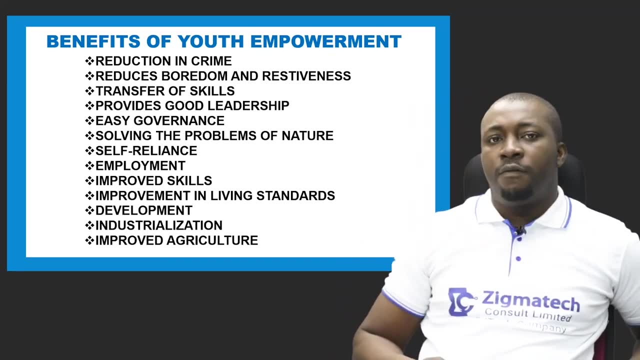 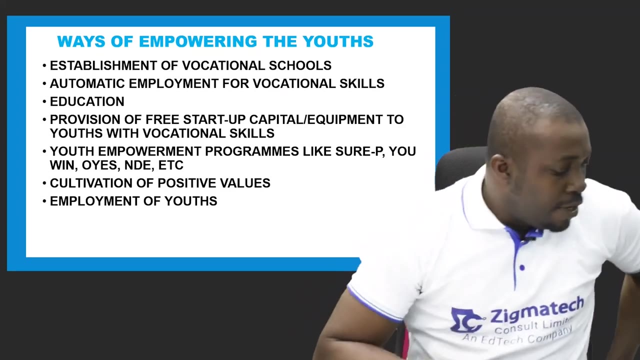 Train people on agriculture through agriculture extension services, soft loans to farmers. Of course, it will improve agricultural development in the country. So these are the benefits and importance and needs for youth empowerment. Now let's look at the various ways of empowering the youths in our society. 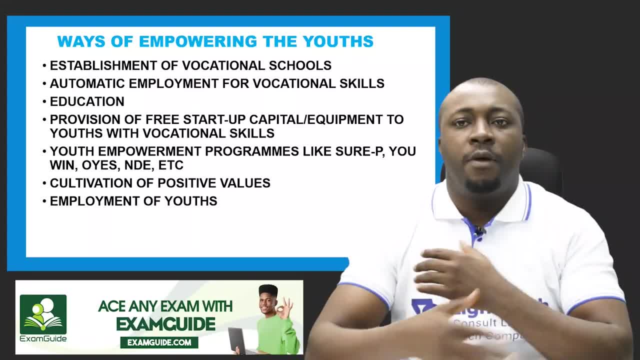 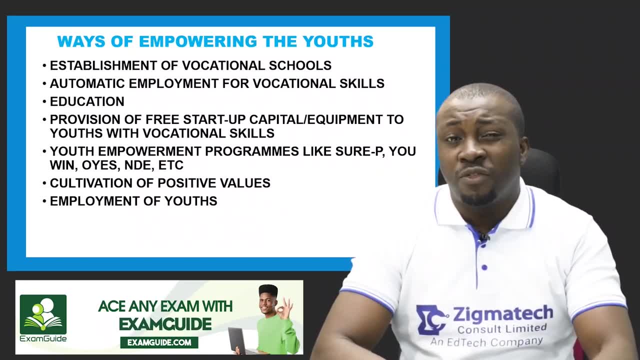 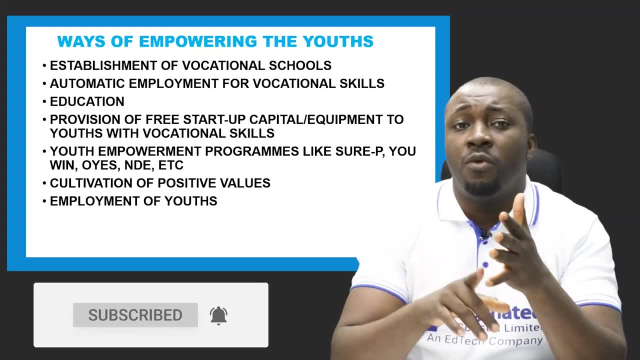 There are many ways to empower the youths, Both the government and groups and individuals. One: establishment of vocational schools. Now there are some schools that are vocational schools Now. these schools train people on various vocations, like sewing, It could be baking of cake bakery. 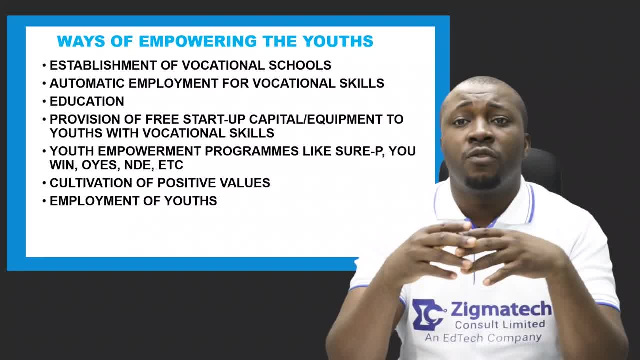 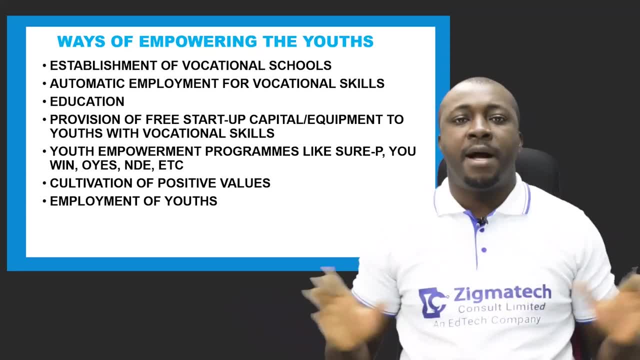 It could be designing one thing or the other. So, establishment of vocational schools by the governments, individuals and groups, We go a long way in empowering the youth, Because it's not everybody that wants to go through the stress of formal education on university level. 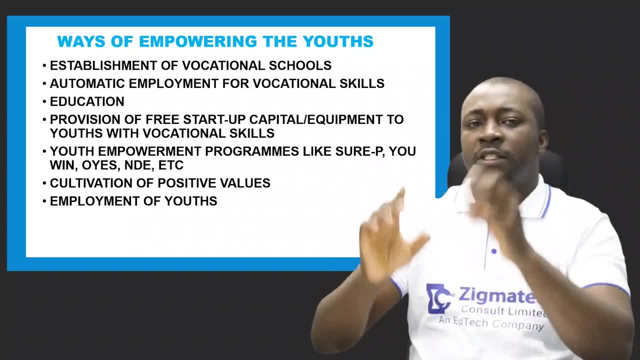 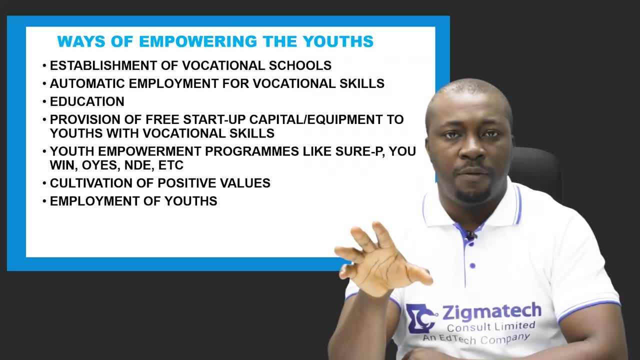 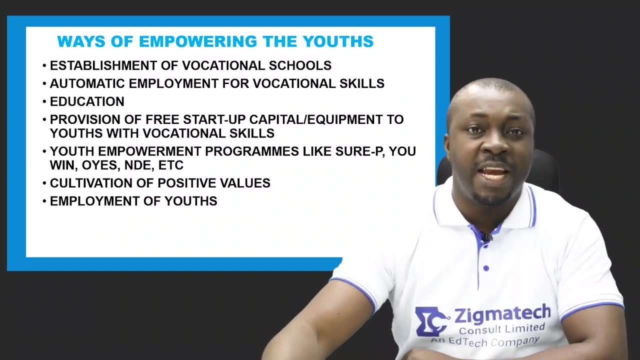 But through vocational schools people can get one skill and start up their means of living. Now, automatic employment for vocational skills. Now giving automatic employment to people with vocational skills to practice the vocation that they have learned or that have been trained on. 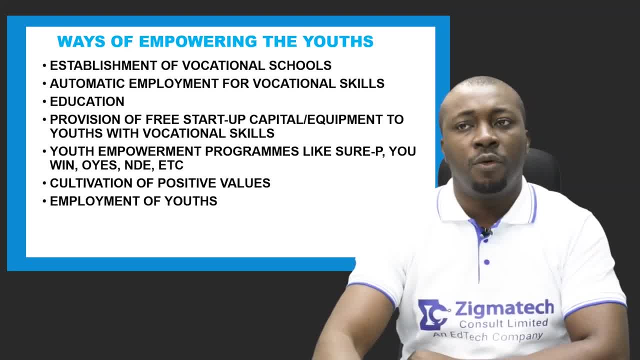 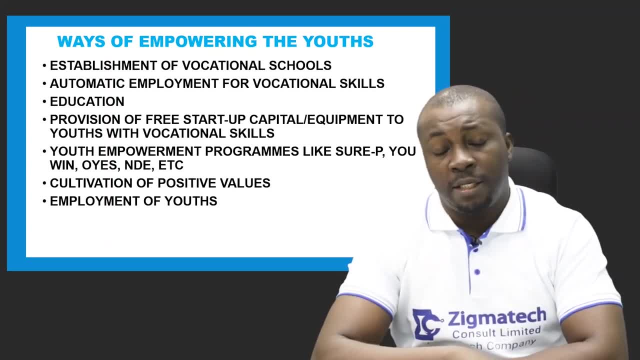 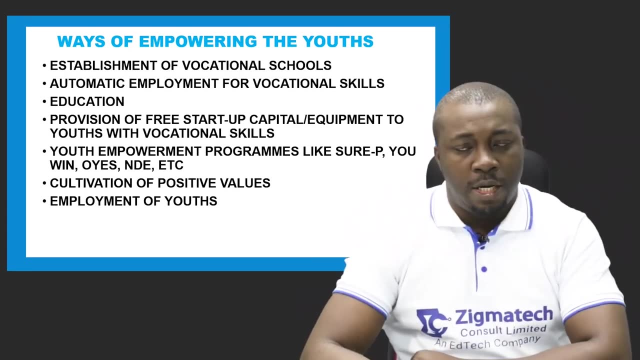 It's another way to empower the youths. When government has such program or individuals and groups. If we have that example- somebody who has learned catering Because, okay, in this hotel, I work there- It can help to empower the youths. 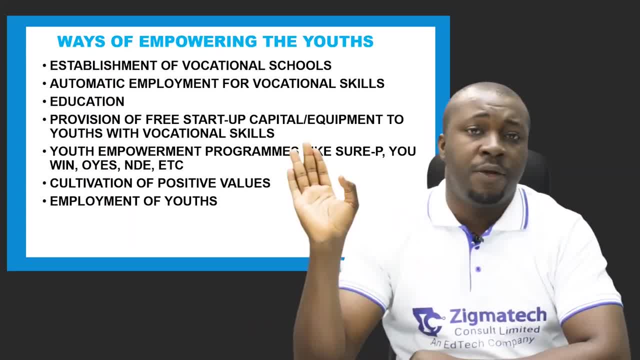 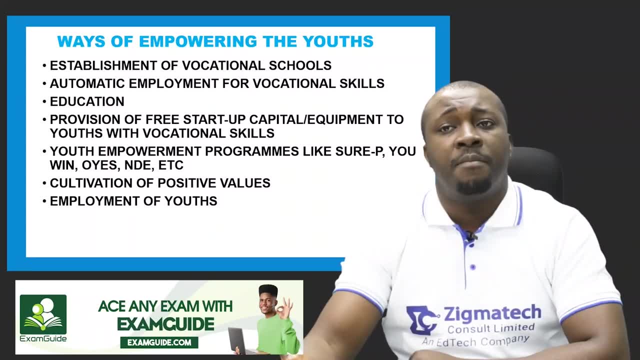 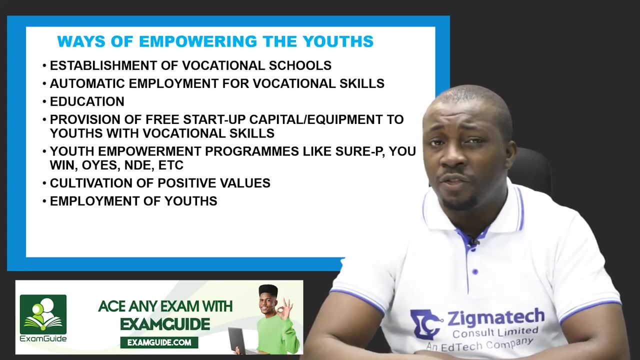 Also, education is number one way of empowering youths, Ensuring there is education to the youths. And how can you make education empower people? People, through education, can make education to a certain level- secondary level, free, Basic education should be free for people. 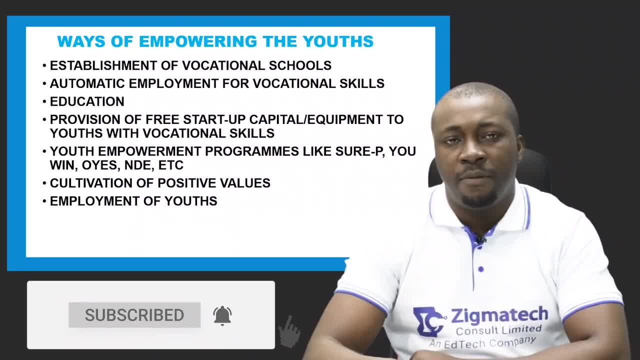 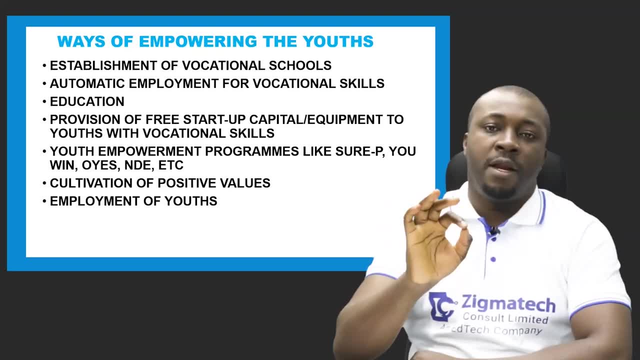 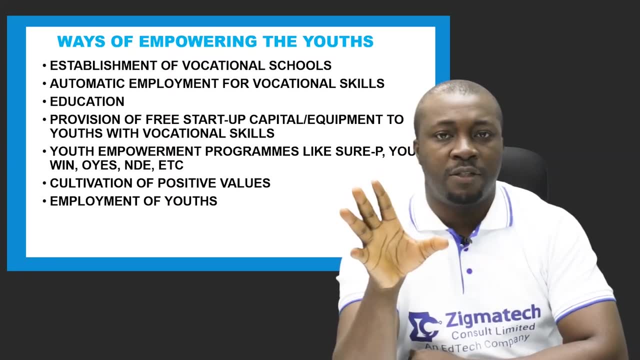 Or government should subsidize it to the barest minimum that people, even the poor, can afford. So it's a surest way of empowering the youth, Because in education people are trained with knowledge skills. They get many trainings through the process of formal education. 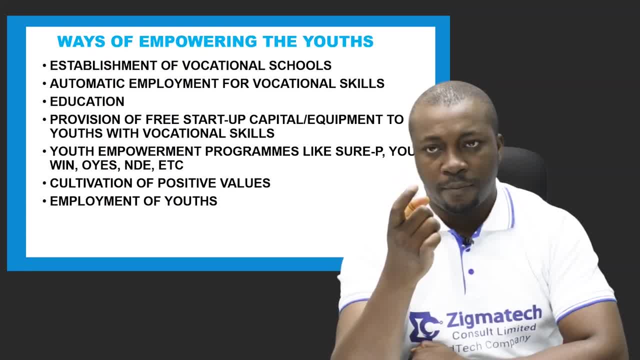 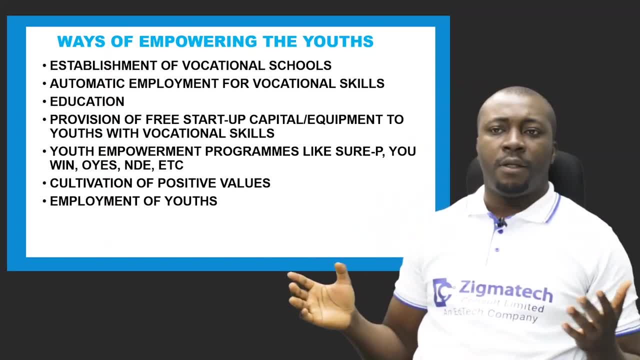 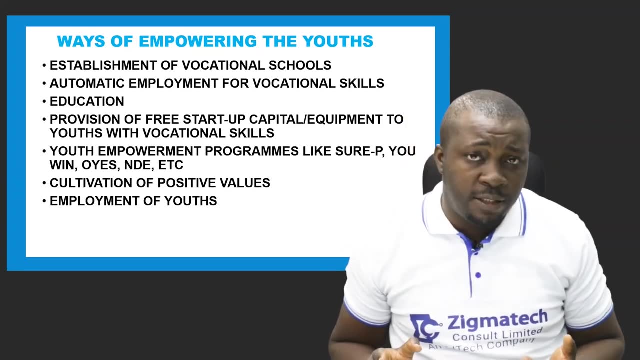 Now provision of free start-ups. Start-up capital Equipment should be used with vocational skills. Now somebody has learned tailoring. May not have the money. You need a sewing machine, You need a shop where you can work And you have to rent it. 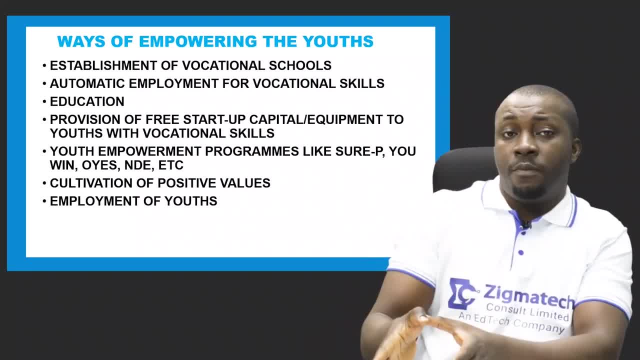 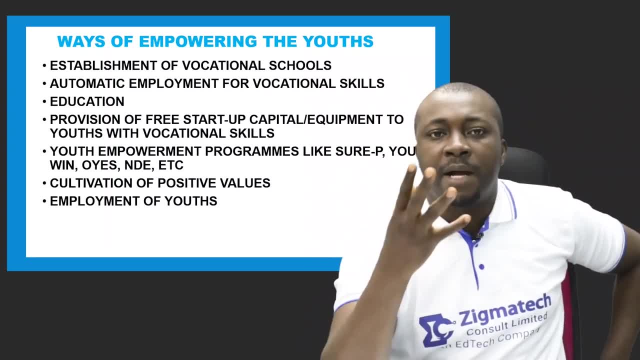 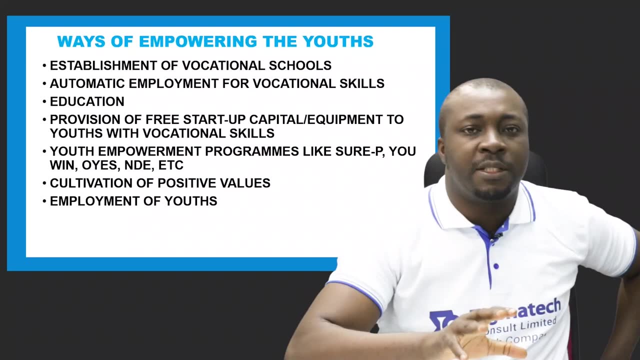 Now, free start-up capital is when government or any group gives somebody free capital to buy equipment Or provide this equipment to the person- Start-up capital. Somebody who's into catering needs equipment. So if you have learned any vocation, the person needs equipment and capital to get this equipment. 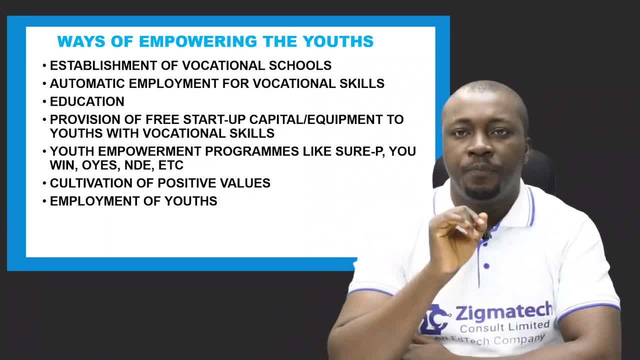 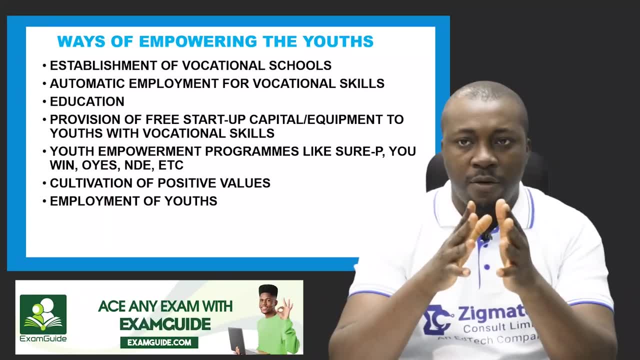 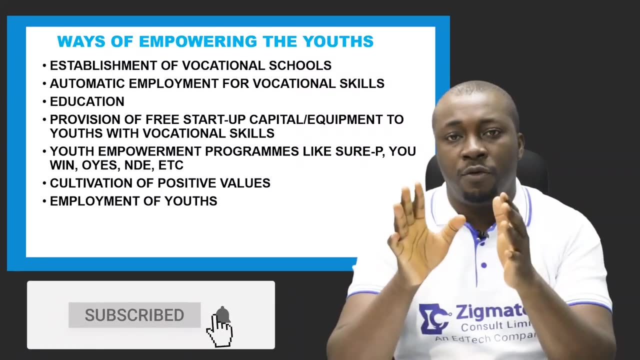 So provision of this equipment can help in empowering the youth. Now youth programs by the government, like SOPE We are going to talk about UN OES, NDE A to C Can also help to empower the youth When government rule out programs. 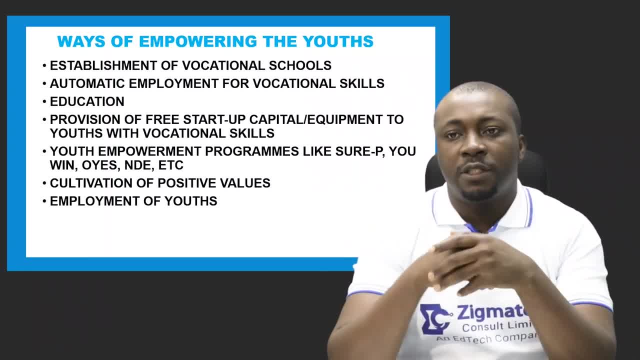 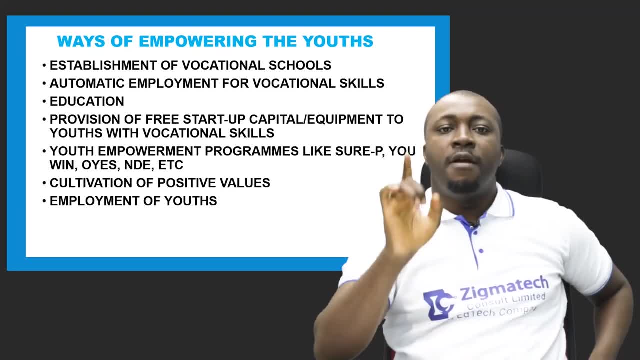 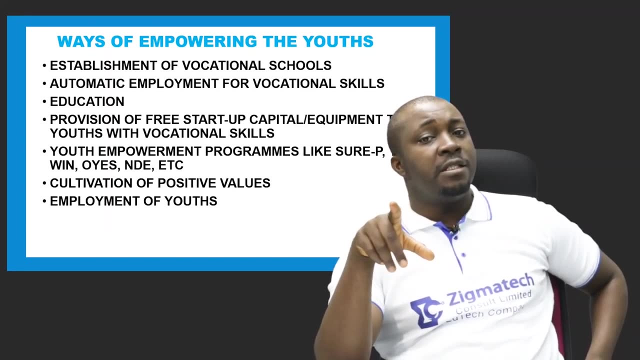 To help empower the youth. It will, of course, help to empower the youth. Then, cultivation of positive values, Values like hard work, Values like self-reliance, Can help to actually empower the youth, And that is why, in civic education, we emphasize values. 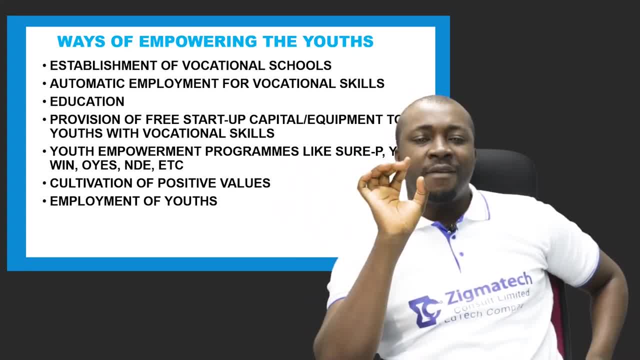 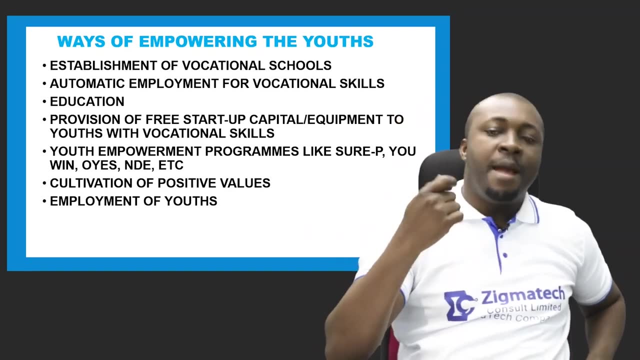 Because we want the young people to have the right values, Especially the value of self-reliance, selflessness, Hard work is a must-have for every youth. So when we cultivate the right values, we are empowering the youth. Then employment opportunities to the youth. 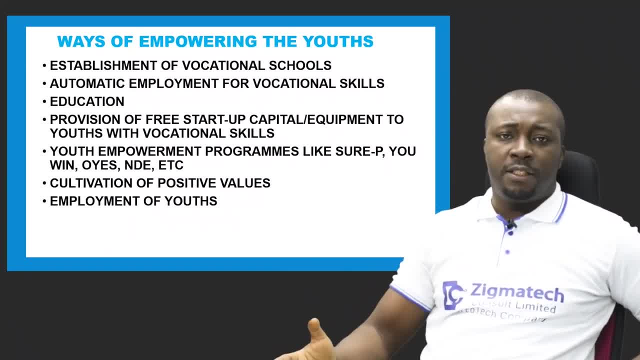 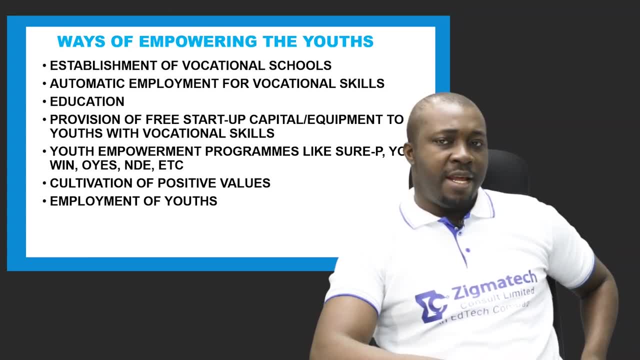 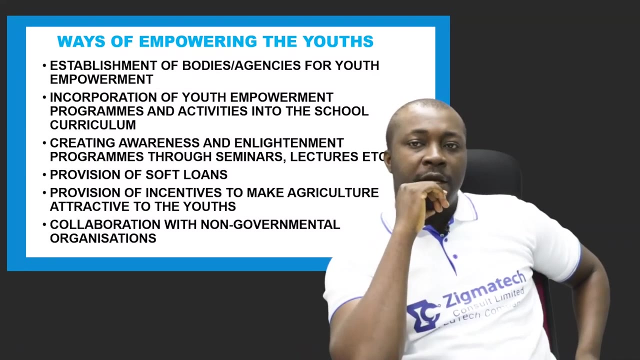 Giving them employment opportunities through agencies of government, Through private establishment. Also, creating enabling environments for employment opportunities Is a way to empower the youth, Of course engaging them by marshalling out these policies Now. we can also empower youth by establishing bodies or agencies. 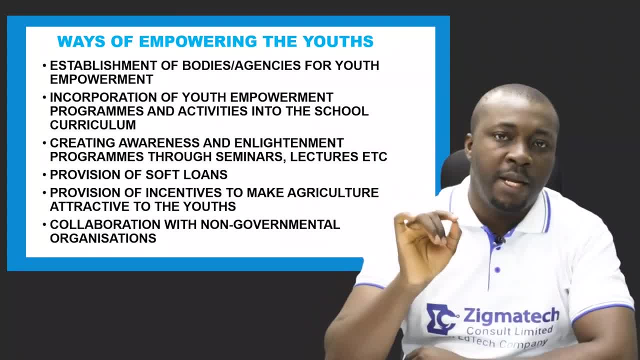 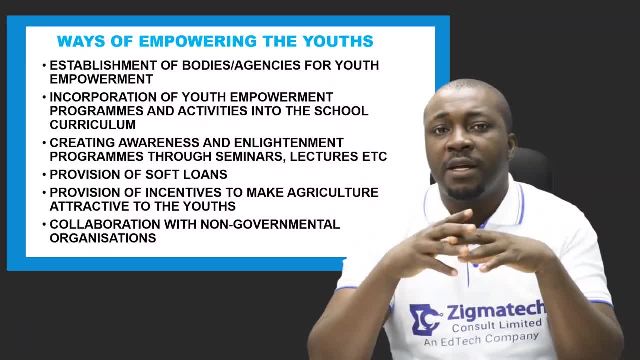 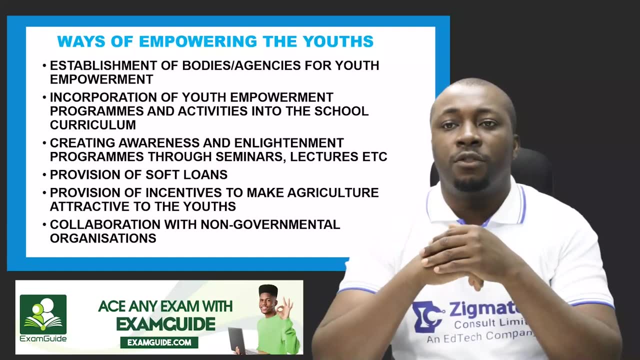 That will be responsible for youth empowerment, That is, the government should create agencies. We are going to talk about it in detail later. Government should create agencies That are responsible primarily to ensure youth empowerment Now also incorporation of youth, Youth empowerment programs and activities in school curriculum. 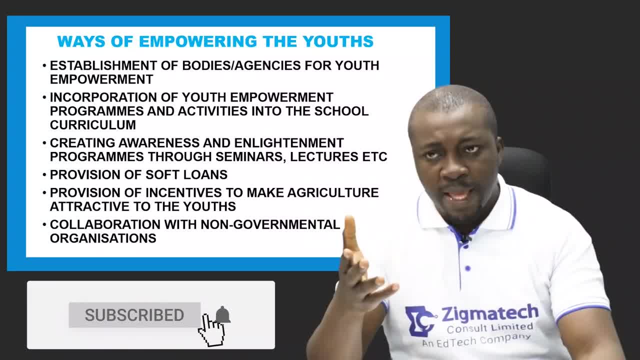 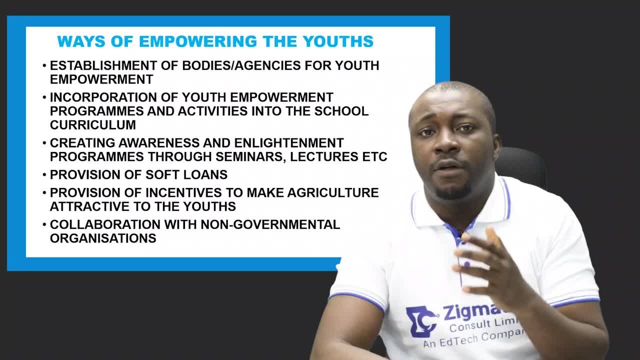 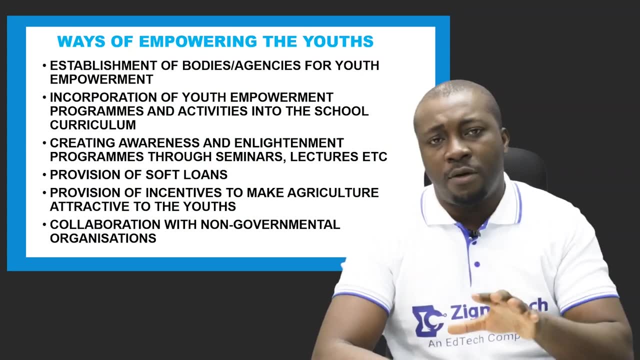 We are going a long way to actually empower youth If we have youth empowerment programs through some subjects And that is why we now have some trade subjects in school, Vocational subjects in school That we help to empower the youth. So incorporation of these things into curriculum. 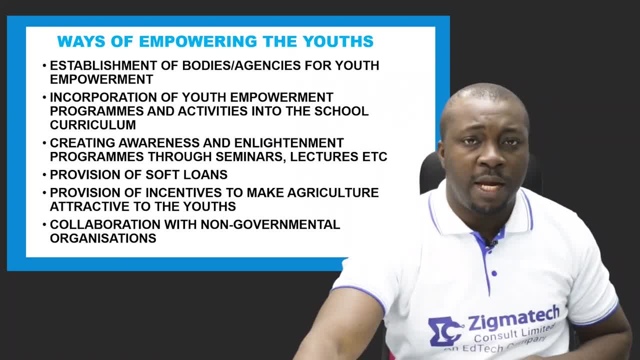 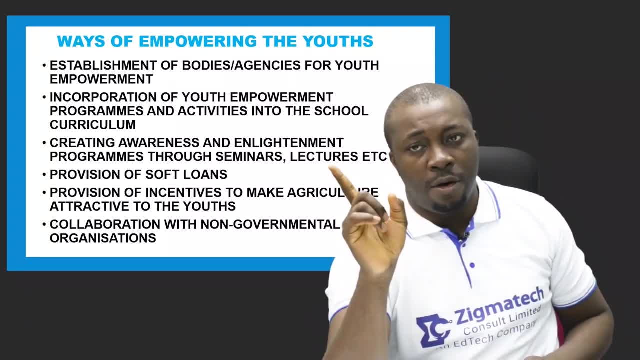 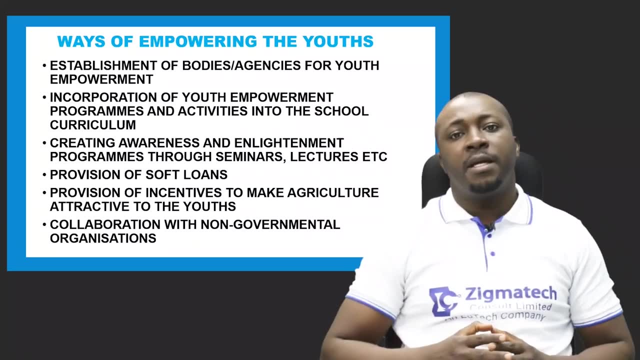 In such a way that anybody that attends formal education in Nigeria or any other country Will be automatically empowered And equipped with one vocational skill or the other. Then also creating awareness and enlightenment programs Through seminars and lectures on youth empowerment Can also be a way to actually empower the youth. 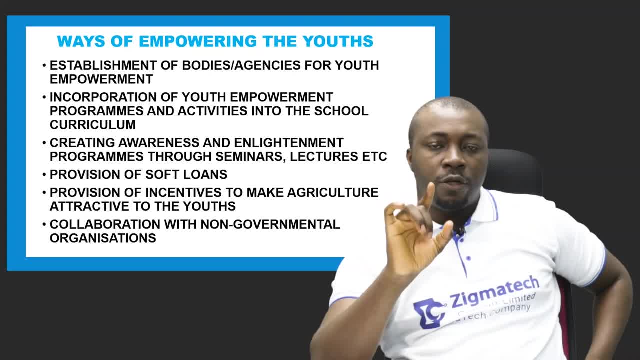 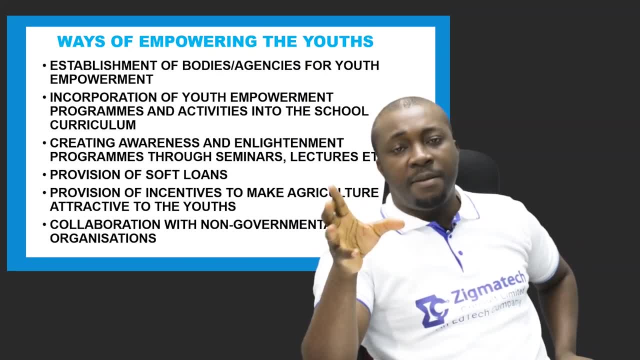 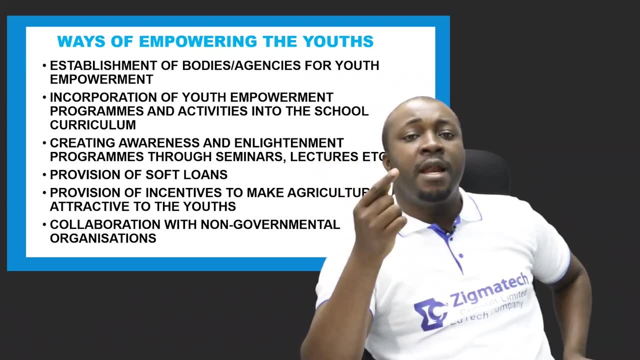 Then provision of soft loans For small and medium enterprises, That is, SMEs, If you give soft loans to youth Because there are people that have skills, There are people that have learned one skill or one vocation, Even trade or the other. 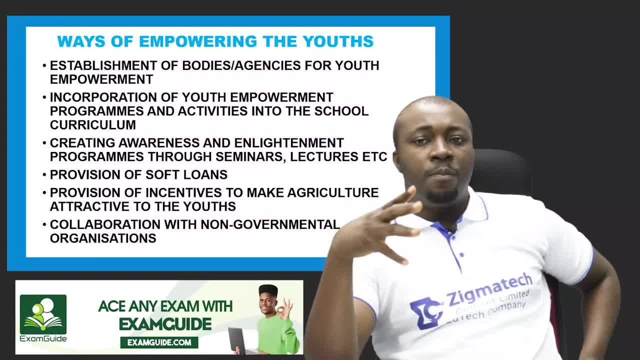 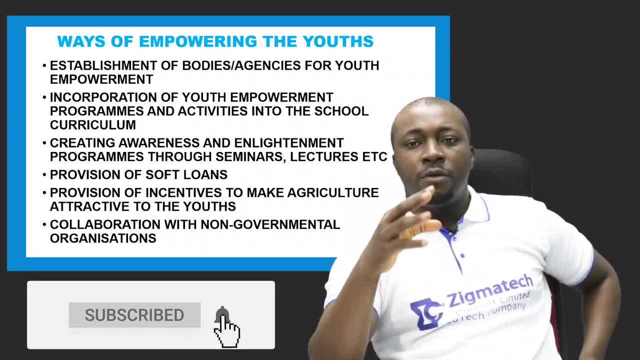 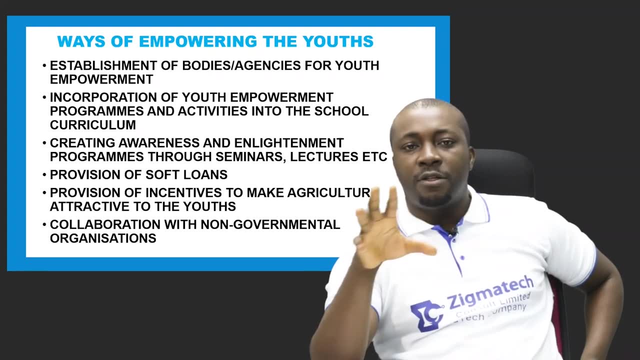 But they do not have the money. So providing them with soft loans- Soft loan is small term loans- Can help to actually empower the youth. Then if we provide incentives to make agriculture attractive- Incentive like subsidizing agricultural equipments, Incentive like education- 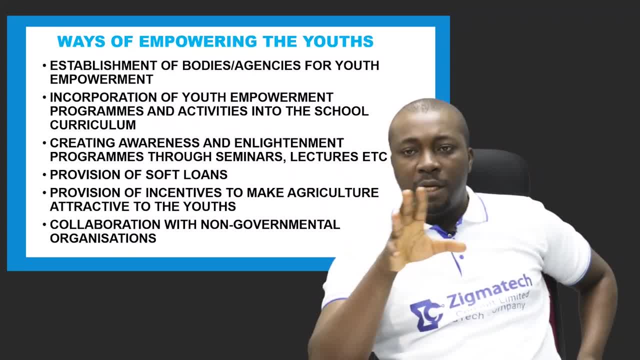 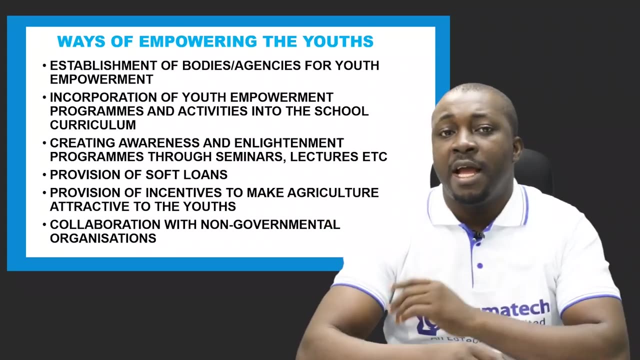 Incentive like soft loans to farmers. It will help to make agriculture attractive, Because agriculture remains the most untapped And under harnessed field, Economic field in the country. The most Because many youths are neglecting agriculture And shying away from indulging in agricultural activity. 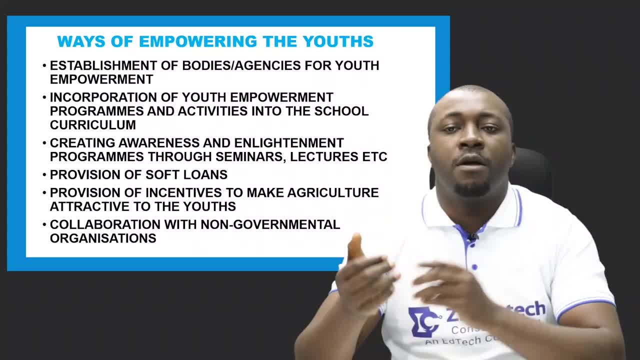 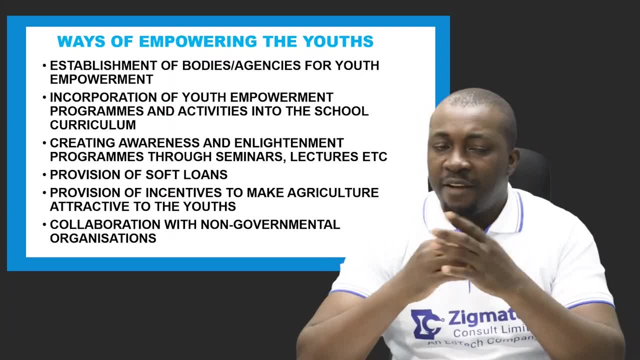 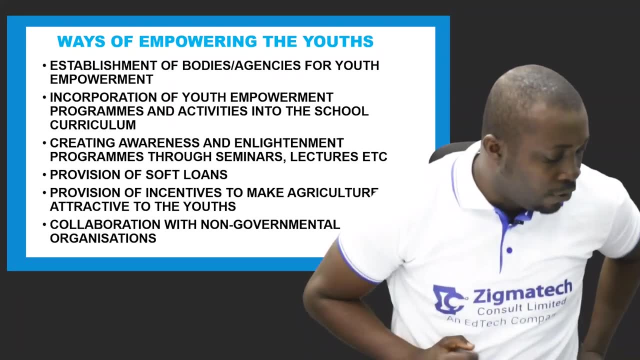 Involving themselves in agricultural activities. Also, government can empower youth by collaborating With non-governmental organizations, Private organizations. Government can work hand in hand with them To see to the empowerment of the youth. Now let's look at some programs and agencies. 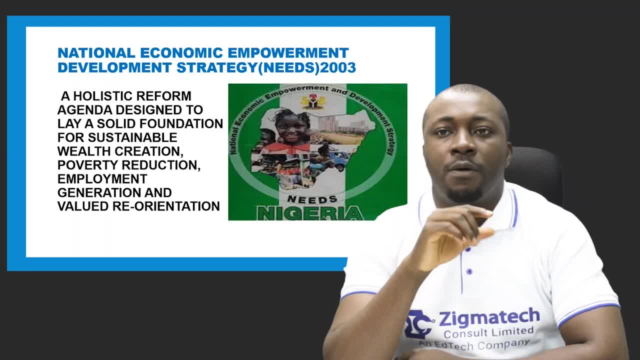 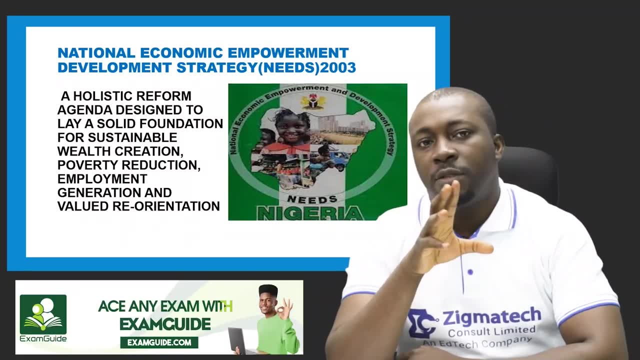 Established to empower the youth. Number one is what we call The National Economic Empowerment and Development Strategy. It was created in 2003. By the government of Olusegu Obasanjo. Now this program is defined as a holistic reform agenda. 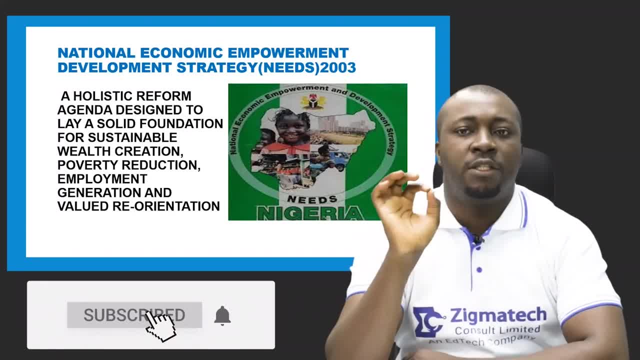 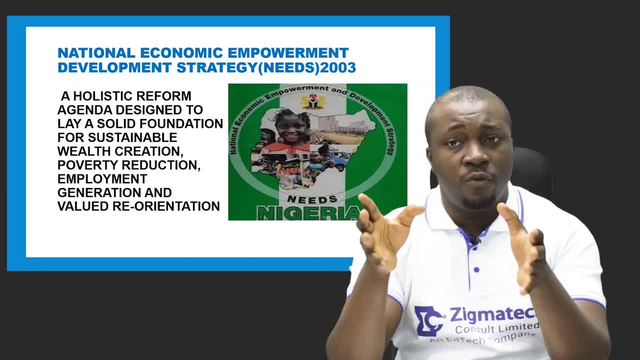 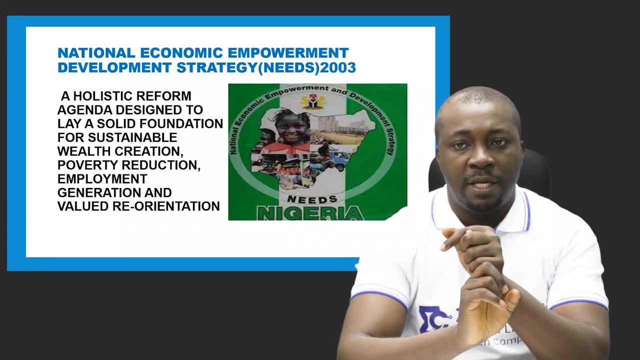 Designed to lay a solid foundation For sustainable one. Wealth creation Is one of the aims of the program, And to create wealth To reduce poverty, And reducing poverty by empowering the youth- Create employment, Employment, generation And also valued or reorientation. 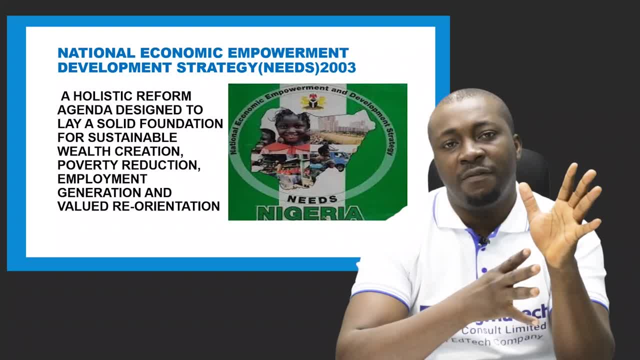 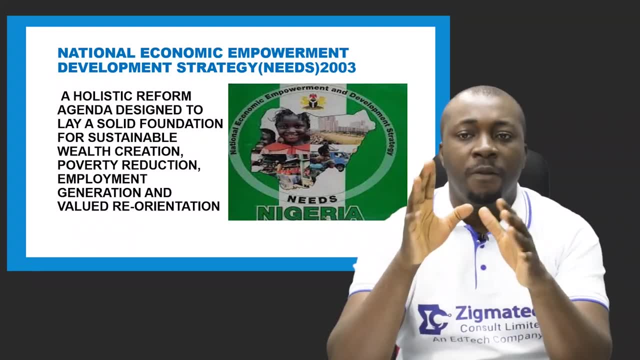 Now to change our value, From the negative value To the positive value. To change our value That one does not need to be patient And work hard in order to make money. So value reorientation. So the needs. 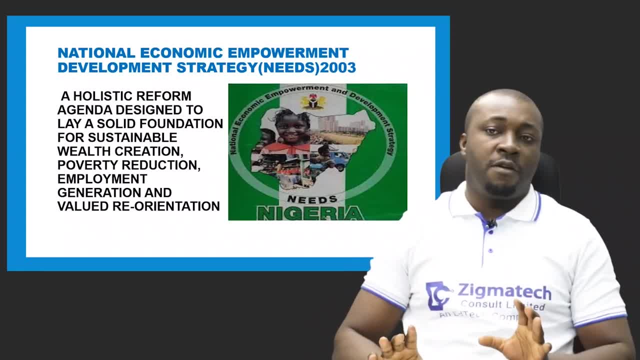 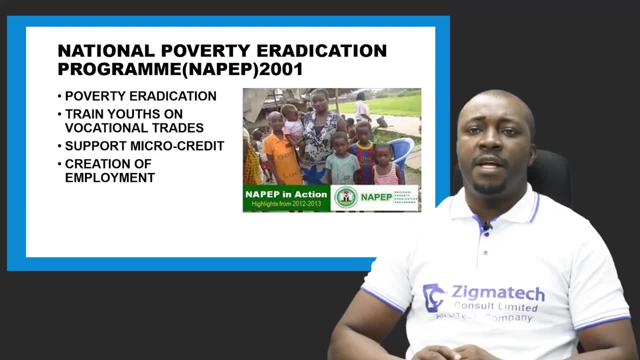 Is an empowerment program Or the federal government Of Nigeria. For these reasons, Now, another empowerment program Of the government of Nigeria Is what we call National Poverty Eradication Program, NAPEP. That was created in 2001.. 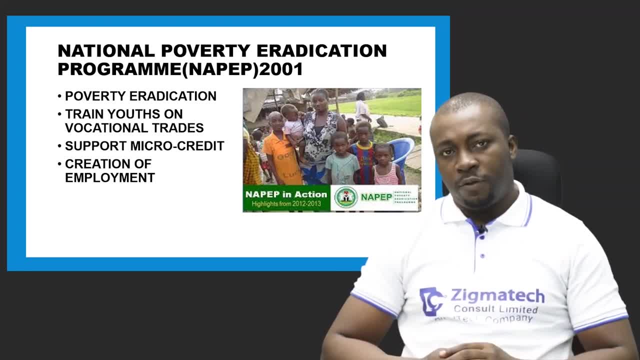 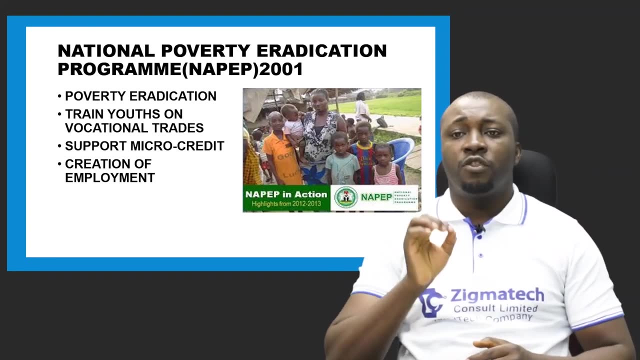 By the government of Chief Olusegu Obasanjo. The aim of the program is Poverty eradication By providing even softer loans And also vocational training of youth, Training youth on vocational training, Then support microcredit. That is soft loans. 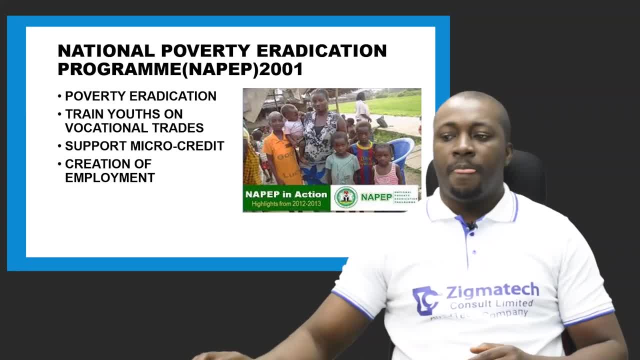 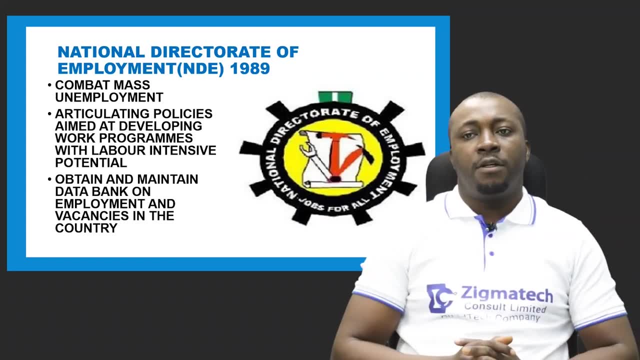 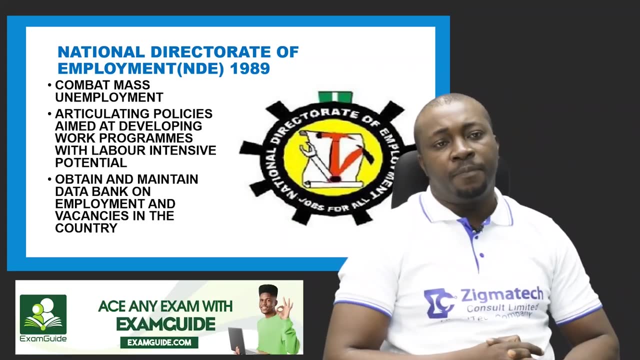 To the youth And the creation of employment. Now we also have another agency of government Called National Directorate of Employment, Which was created in 1989. By the military government Of Abraham Badamosi- General Abraham Badamosi. 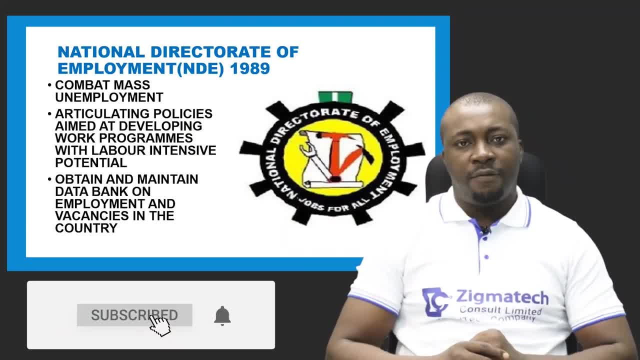 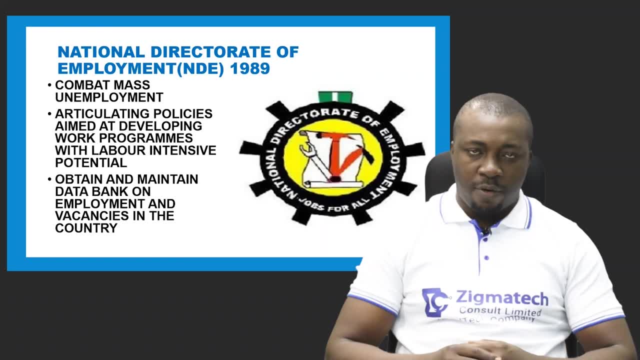 Babangeda Now, the aim of this agency, The reason for its creation, Is to combat mass unemployment And see to it That we are sufficiently employed In our country, Articulating policies Aimed at developing work programs. 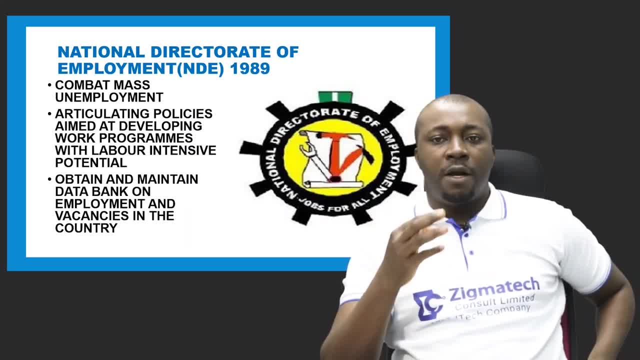 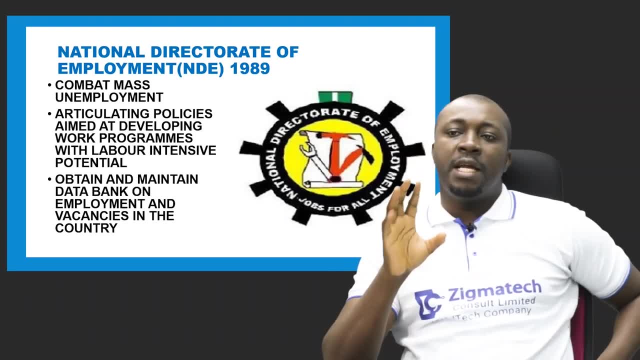 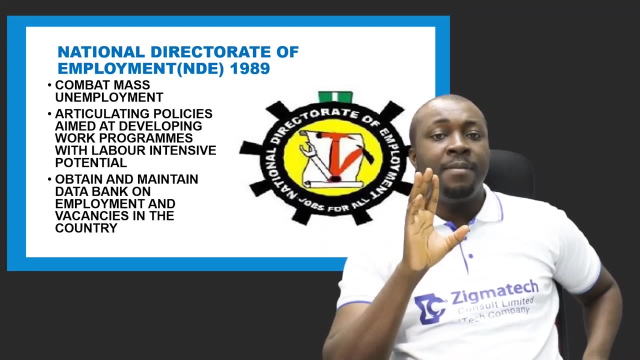 With labor intensive potentials. Another aim is to obtain And maintain data back On employment and vacancies In the country. Now it is this agency That keeps data And statistics On the employment And unemployment rate Of the country. 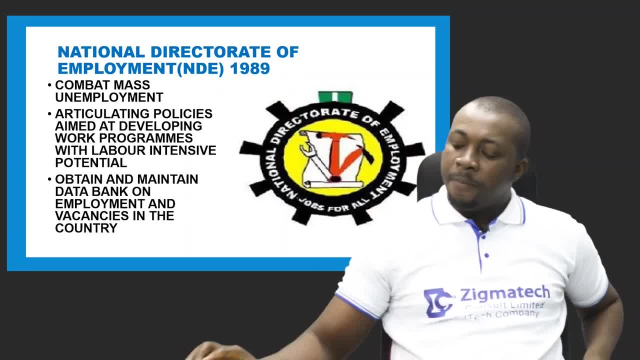 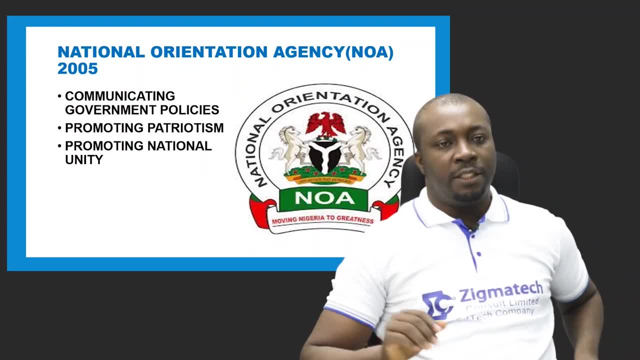 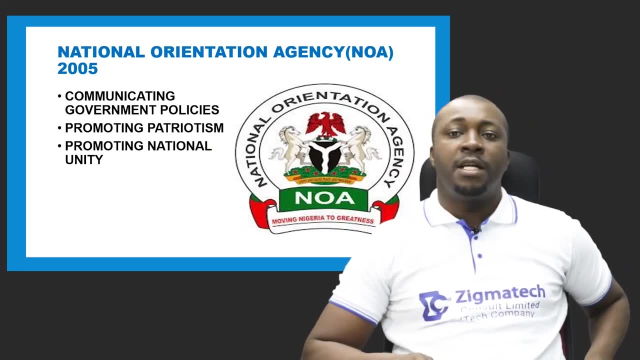 And also helps To advertise vacancies In the country. Another agency We are going to talk about Is National Orientation Agency. That was established in 2005.. National Orientation Agency Was also established By the government of Chief Olusegu Obasanjo. 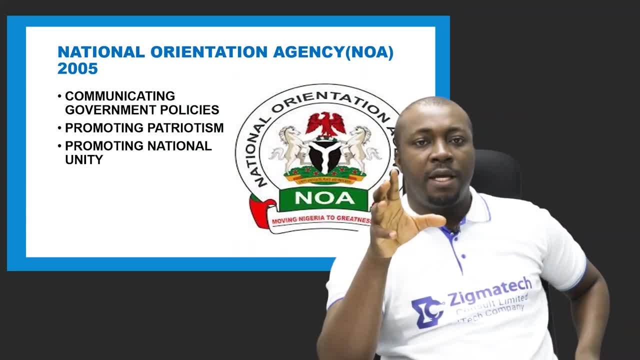 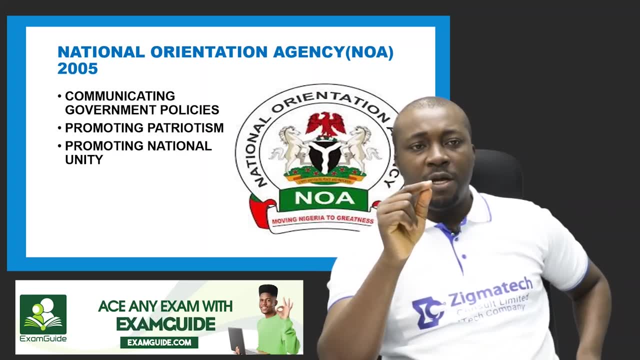 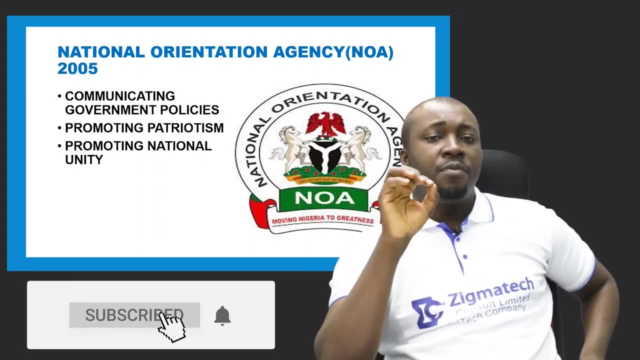 Now the aim of this? It empowers the youth By communicating government policies To the people, Giving proper orientation Of people About the government policy, Promoting patriotism Among people And promoting national unity In the country. Another government program. 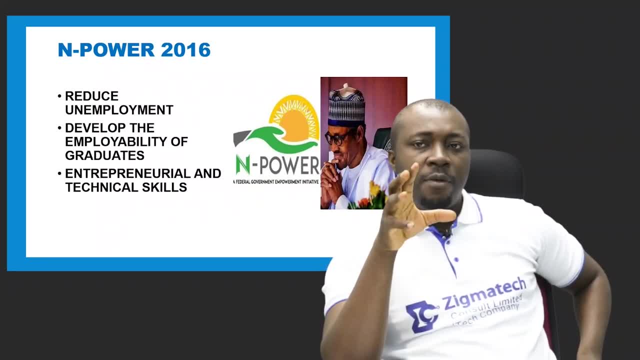 Aimed at empowering the youth Is the program Of the current government In 2022.. Government of President Muhammadu Buhari. That's what we call The empire In 2016.. Now, this is a program. 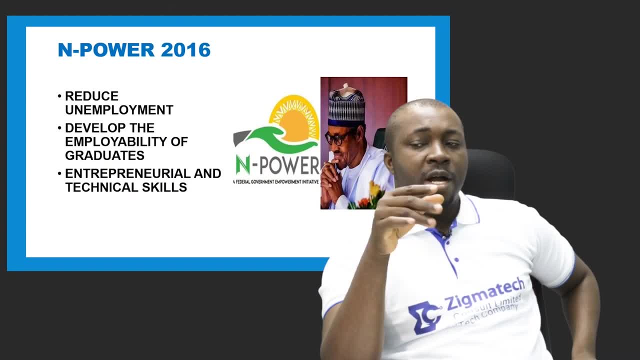 That aims to reduce Unemployment, Because people We have to serve The government, Work in any area Assigned to them By the government And get paid By the government, And then working in those areas They are actually. 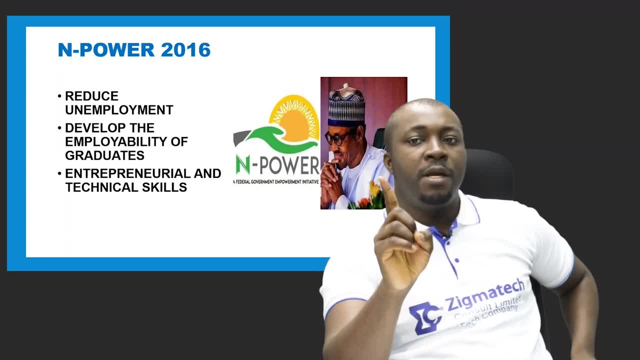 Equipping their skill And employability. So This unemployment Numbers Develop Employability Of graduates Because at times Graduates Are faced With the challenge of After graduating Because they don't have work Experience. 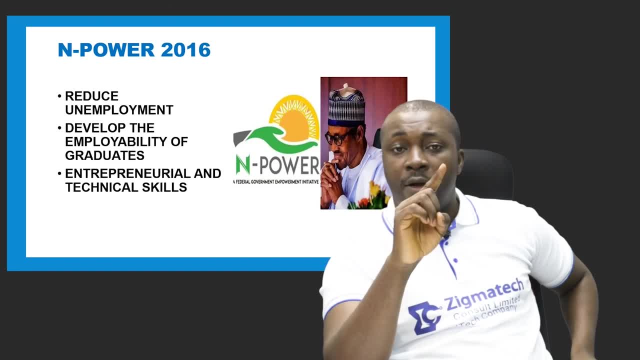 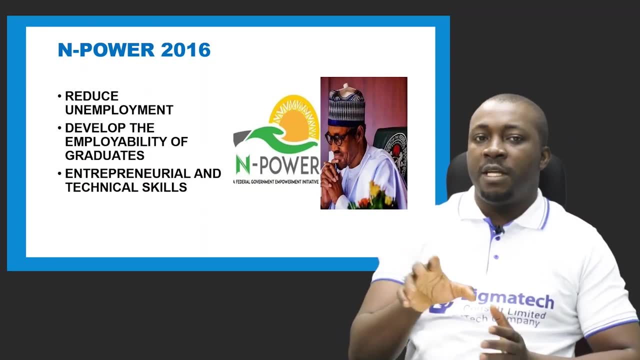 And any skill They may Become, Un I mean, They may become Unemployable. So This scheme Empire Aims to boost The employability By giving them The chance, Opportunity To work In a particular place. 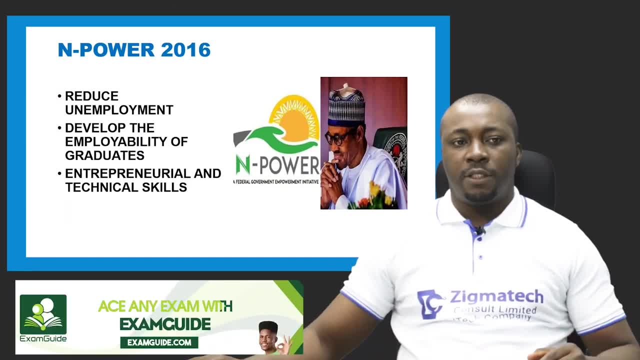 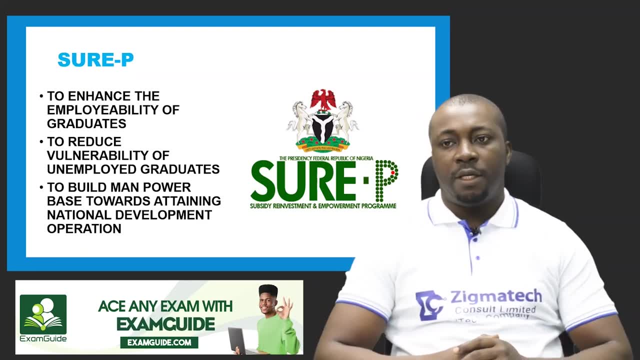 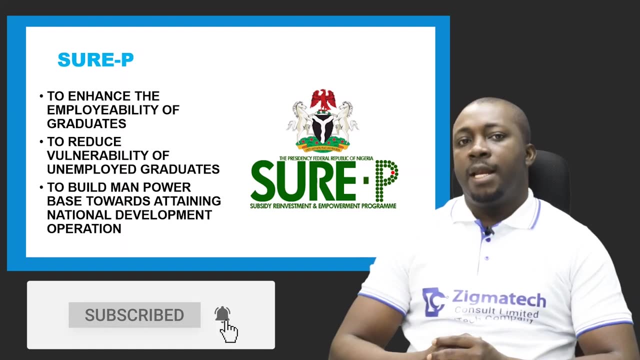 And to improve Their skills And to improve Their professional And technical Skills In Graduates. Then We also have The Shop P Program, That is Subsidy, Reinvestment And empowerment. 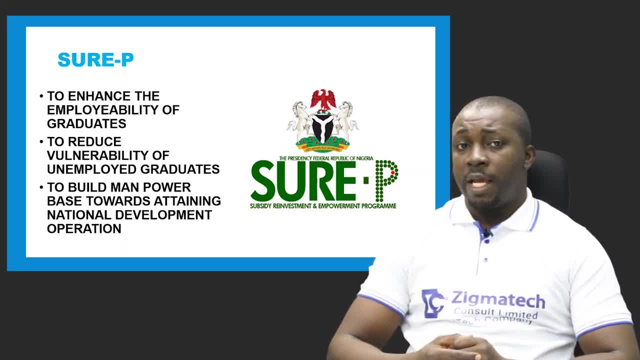 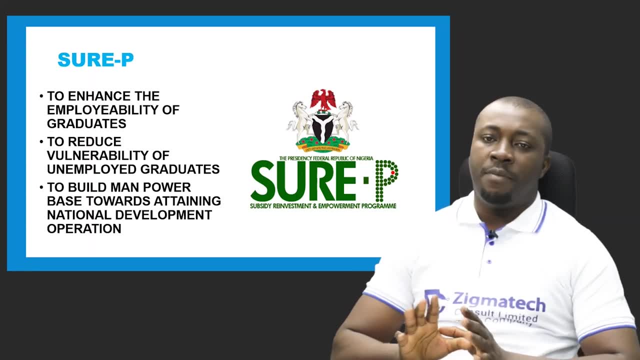 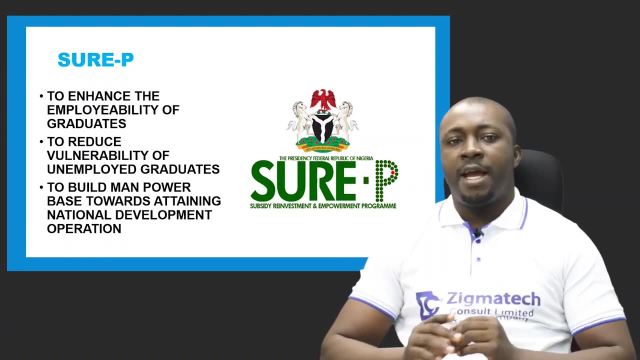 Program Of the government Of Dr Goodluck Ebele Jonathan. Now, This Scheme Was The Employability Of Graduates. Is Is Like The Empire Program, So 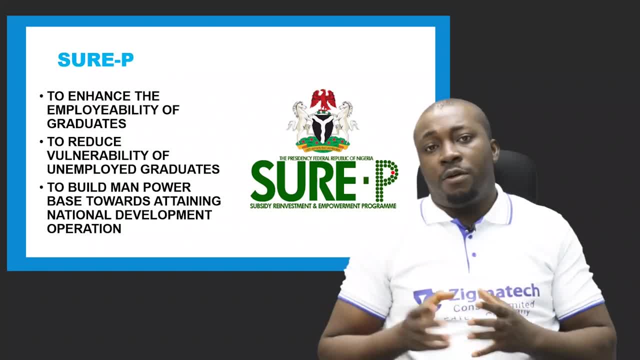 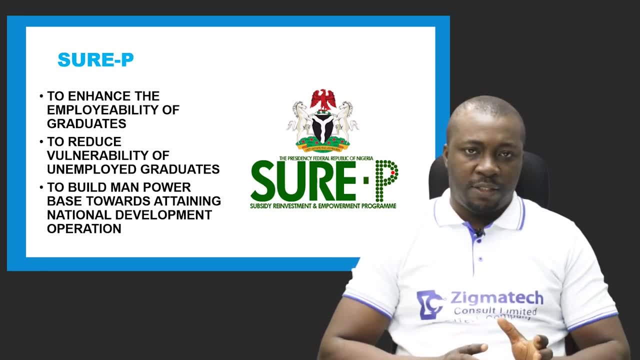 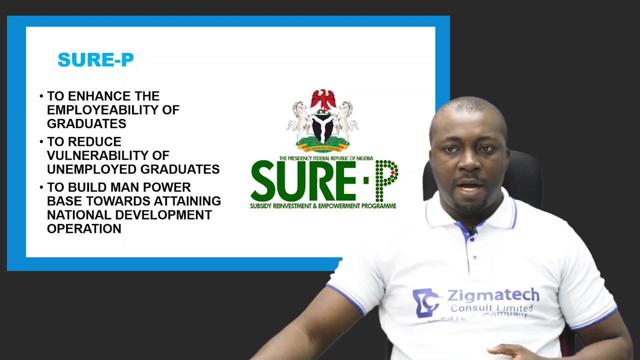 The Graduates Are Expected To Work In The Places That Assigned, That Assigned By The Government, And Get The Employability Of Our Students. Thank You. 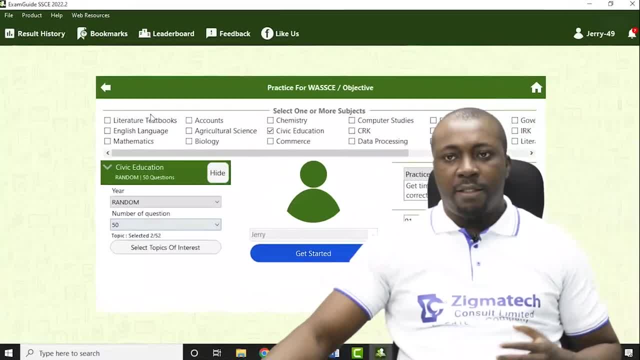 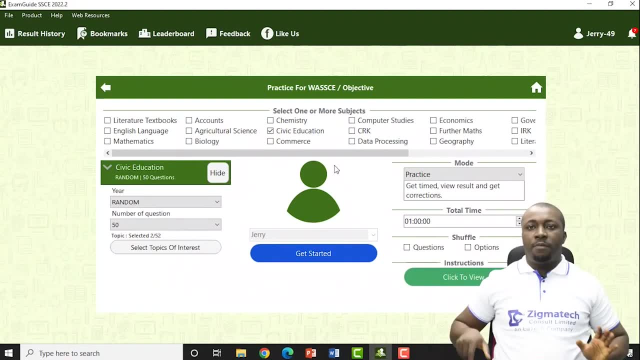 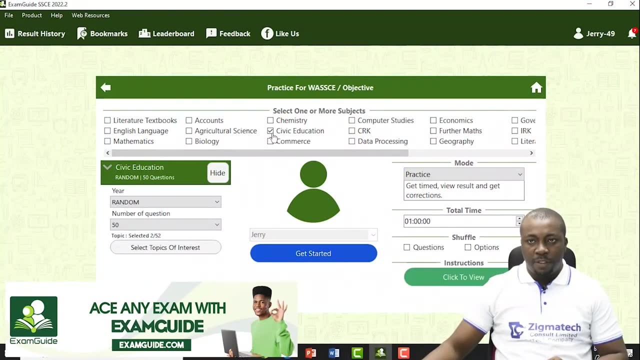 Now We Are Going To Our Practice Session Using Our Exam Guide. Now, This Is Our Exam Guide. We Want To Practice. We Are Not A. 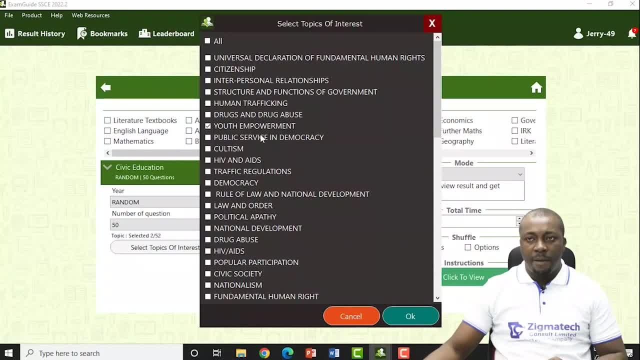 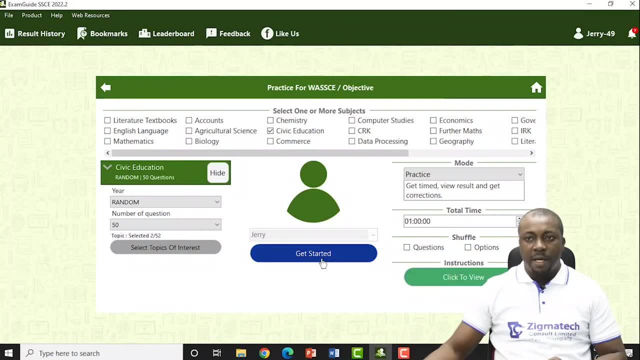 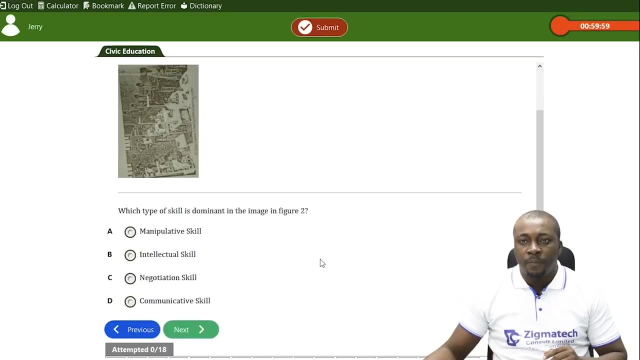 Particular About The Year. Now Topic Of Interest: We Have Selected Youth Empowerment And Also We Have Where We Have Empowerment, So We 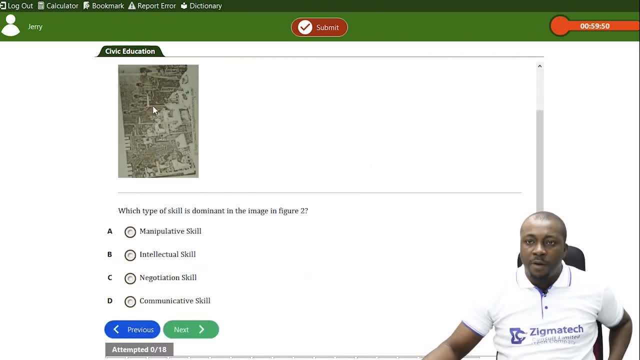 Selected Click Okay, This People Are Into Tellering. Now Tellering Falls On Their Manipulative Skill. They Are Using Their Hand. Make Things. Now The 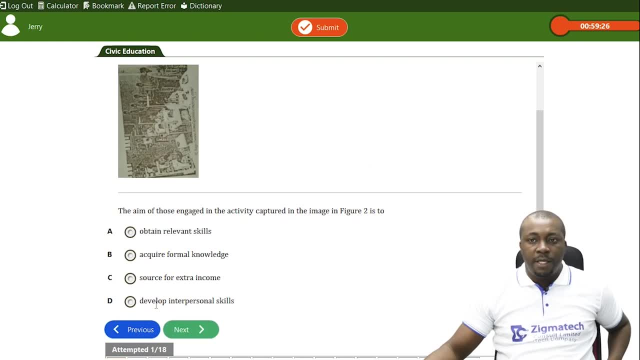 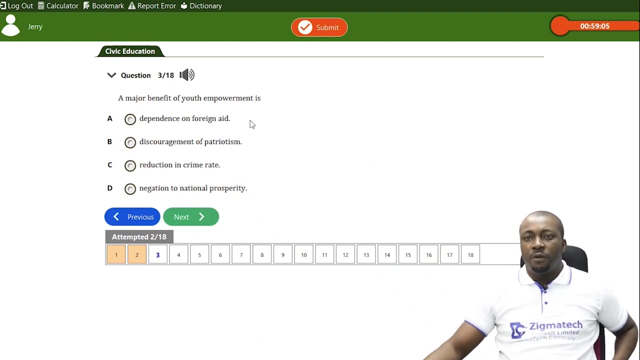 Aim Of Those Engaged In The Activities Capture The Activity Is To Actually Develop Relevance Skill That Will Make Them To Source For The Income. 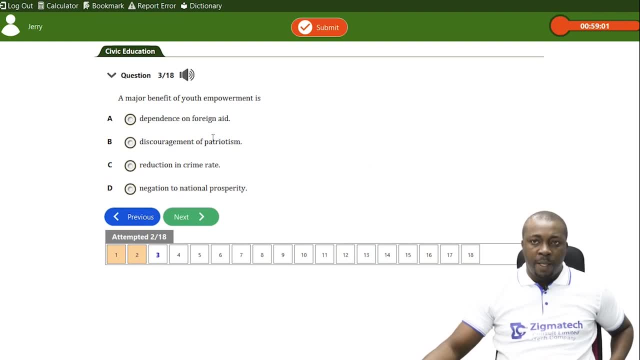 Extra Income Or Income So Relevance Skill That Will Make Them To End. That Is The First One We Discussed. So It Reduces Crime. 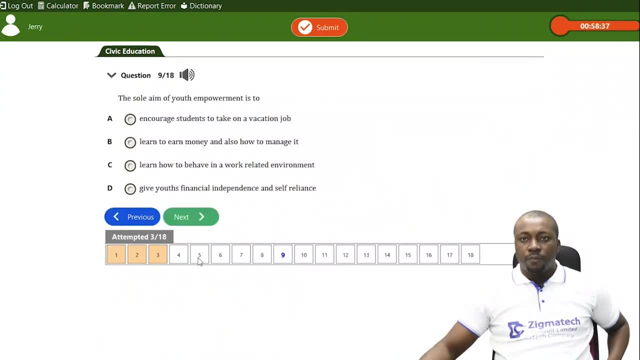 Now Let's Look At Looking For The Short One Now. The Sole Aim Of Youth Empowerment Is To Income B Learn To Earn Money. 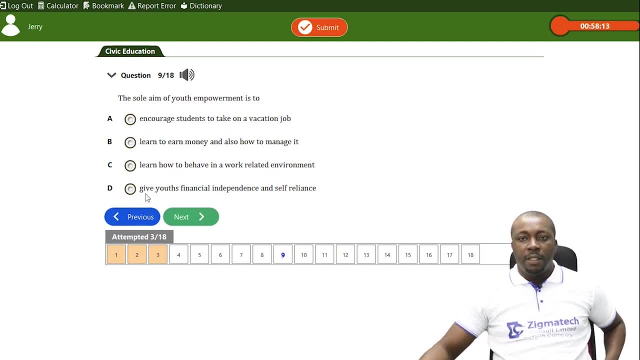 And Also How To Manage It. C- Learn How To Behave In A Work Related Environment. D- Give You Financial Independence And Self Empowerment. 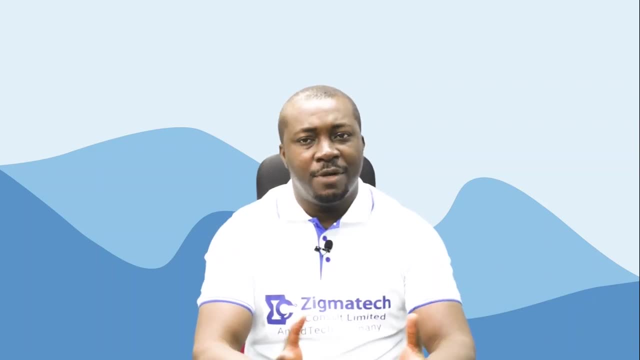 Thank you For Participating In Today's Class. You Can Practice More Questions Using The Exam Guide App. The App Scores And Gives A Detailed Explanation. 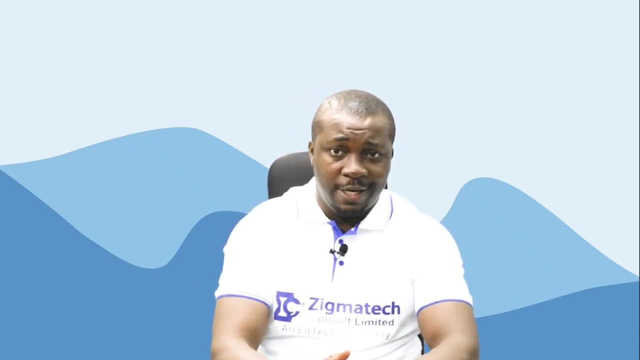 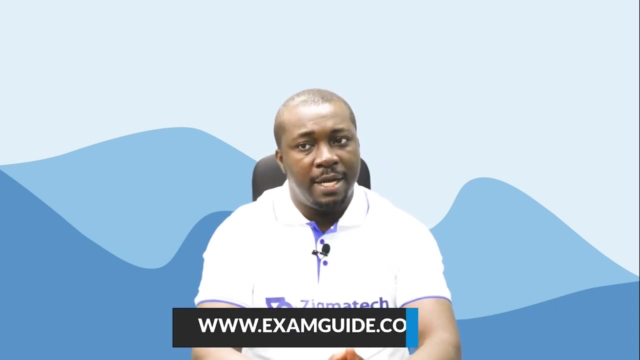 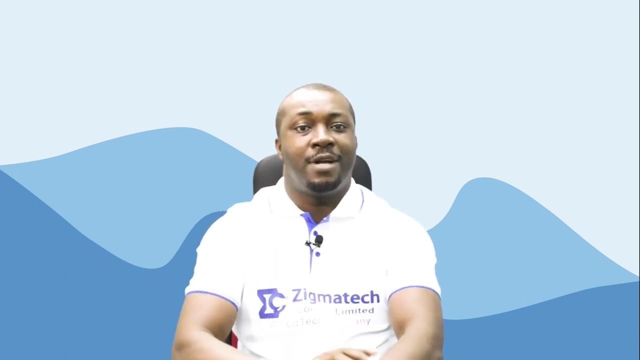 Of All Questions At. It Is A Must For All Serious Students. Download From wwwexamguidecom. If You Don't Have It Yet, See You In.